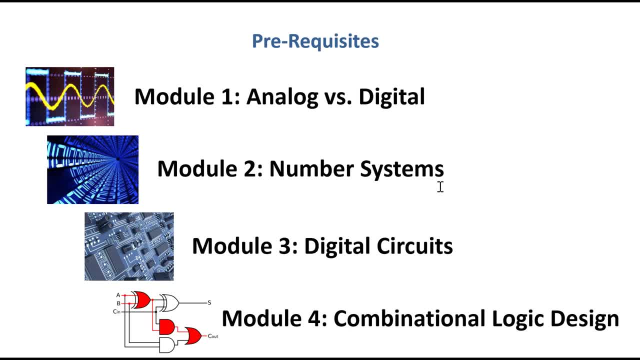 So then we learned about the number systems. So we learned about, instead of using decimal to represent information as a number, we learned the binary number system. And that was because computers are built with, basically, switches, So a switch can either be on or off, and that can produce two discrete voltage levels. 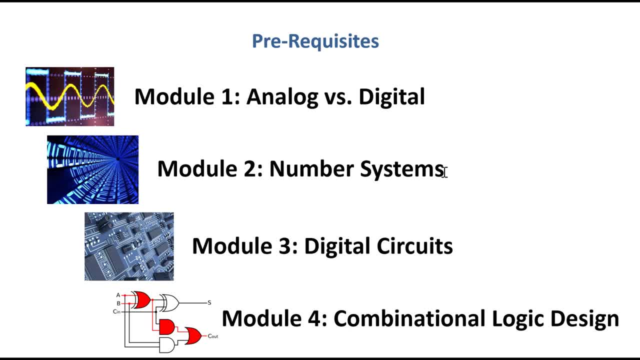 And what we do is we use those voltage levels to represent a number- one or a zero- And then we combine those to create larger and larger numbers, which represents more complex information, And that's how information is acted upon within a computer, Within number systems. we looked at things like representing groups of ones and zeros using the hexadecimal number system. 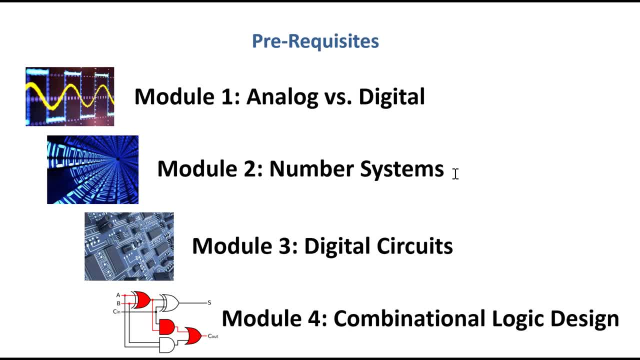 We looked at basic binary arithmetic such as addition and subtraction, And then we looked at representing negative numbers using two's complement. You should also remember module three, which was on digital circuitry and interfacing. This is where we looked at the basic logic operations, things like ands and ors and nays. 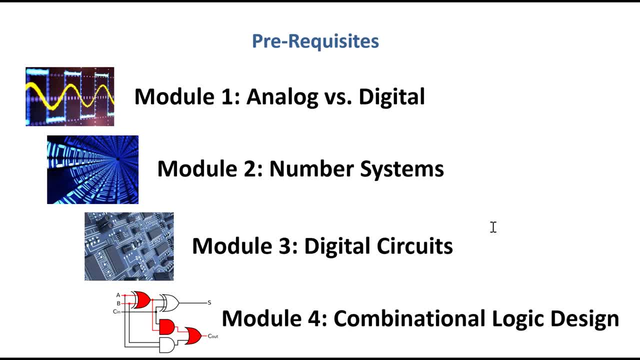 and we looked at their true tables and how they produced an output based upon inputs. but it was all a logic value, And what we mean by logic value is that the inputs to a digital circuit are going to be either a zero or a one. 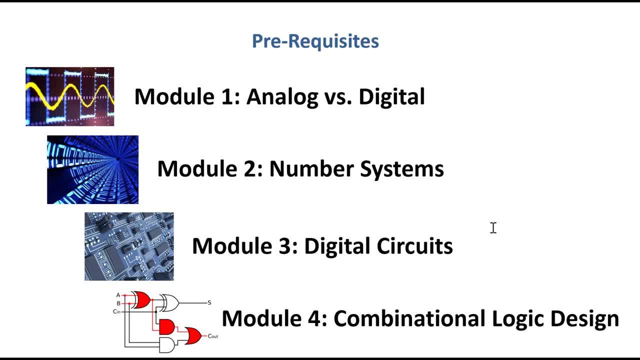 and then the circuit is going to compute the output, which will also be a zero and one. So when we think about a logic gate, that's the basic operations that can take place on ones and zeros and produce an output. But we wanted to actually build hardware. 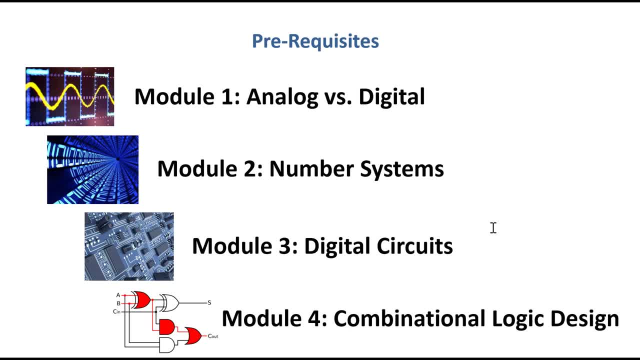 So we needed to look at how do you create these basic gates in the real world, And so we actually looked at discrete parts from the 74 HC series and we were able to put these parts down on our breadboard and actually build basic logic circuits. 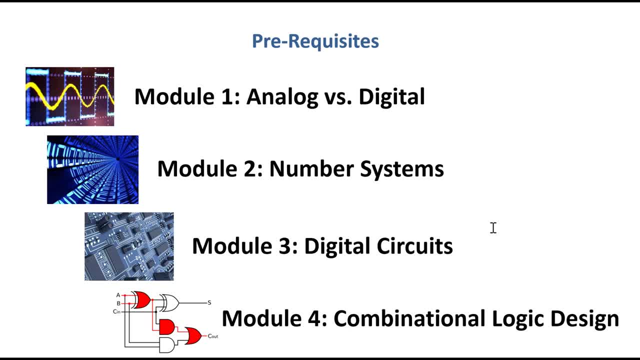 Now, when we started building real circuits, we had to consider the real implementation of these circuits. So we had to consider things like power supplies and grounds. So these logic gates, they don't work unless you provide them a VCC voltage and also a ground. and we also needed to look at the interfacing between gates. 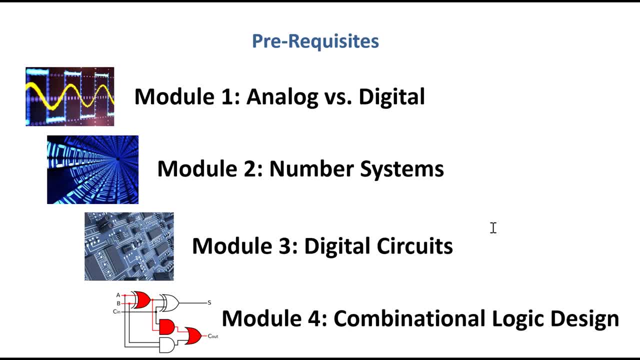 So if one gate is going to produce a logic one and it represents it as a certain voltage level, the gate that receives that information has to be able to interpret that voltage level as the logic one. So we needed to be able to design circuits that can interface with each other. 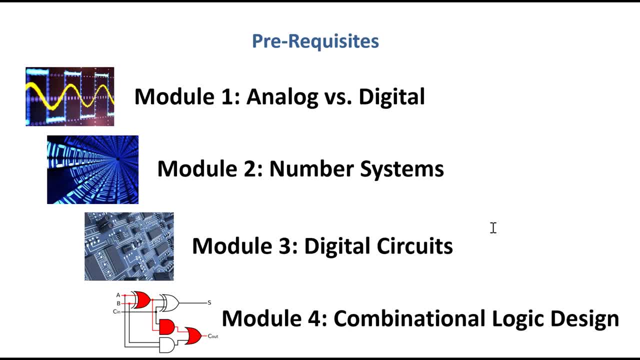 and we needed to be able to understand the operation of these gates in order to interface them properly. So we needed to look at their data sheets. So we looked through their data sheets and we looked at a whole bunch of characteristics about these parts. 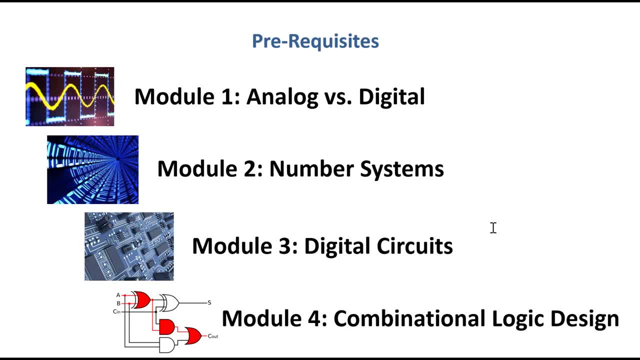 and we also looked at both DC characteristics but also the AC characteristics, so how fast they switch. So once we had all these basic gates in hardware and knew how to interface them, we started looking at combinational logic design. So combinational logic design is where you build circuits that produce a logic output. 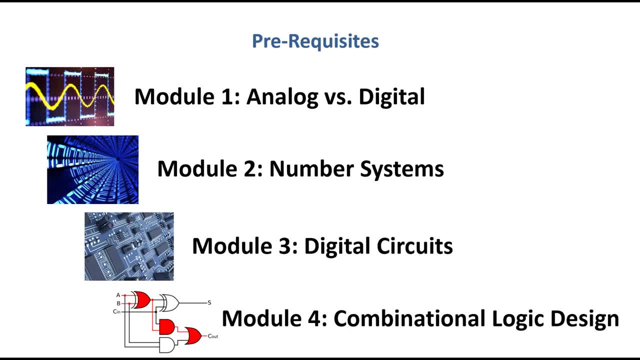 and it's usually just one bit based upon multiple inputs. so two inputs or more, but they were more complex than a basic gate. So instead of an AND gate that had two inputs, you might build a circuit that could implement any arbitrary truth table. 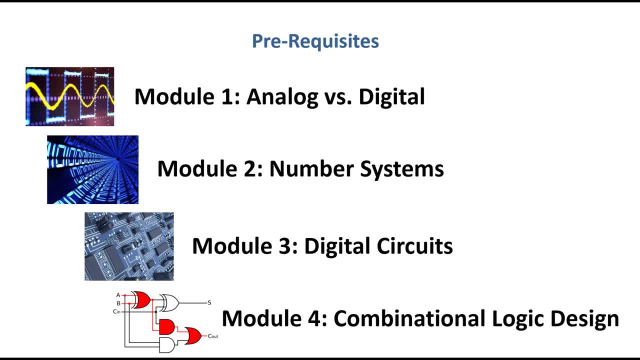 3-input, 4-input, 5-input, truth table, and we learned about how you actually synthesize the circuitry to produce the desired output. Within Module 4 we also looked at minimization, So we looked at how you can build a logic circuit to produce an output in many different forms. 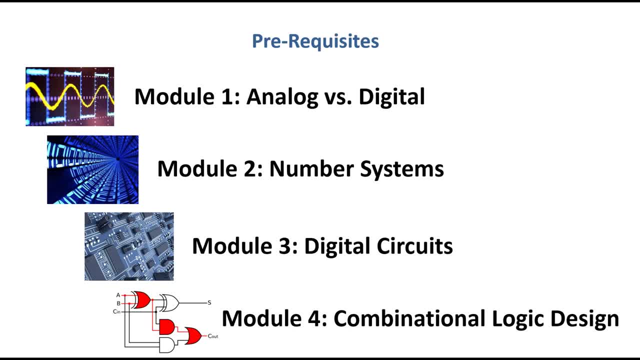 There are a variety of different topologies that you can use to produce the same output, So we looked at how you can build a logic circuit to produce an output in many different forms. There are a variety of different topologies that you can use to produce the same output. 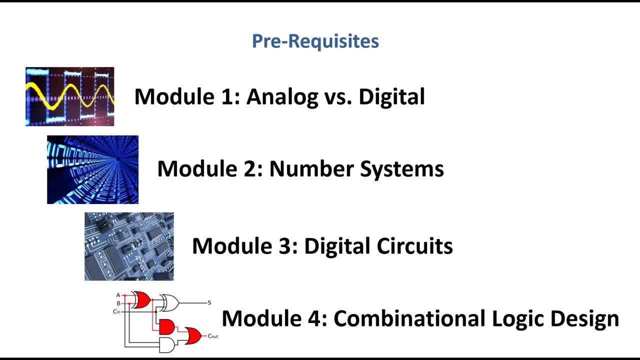 So, depending on what you're trying to do, you might want to choose one topology over another. So that was module four. So if you think back to module four, you think about things like the canonical sum of products, the canonical product of sums, a minimized sum of products using a carnal map. 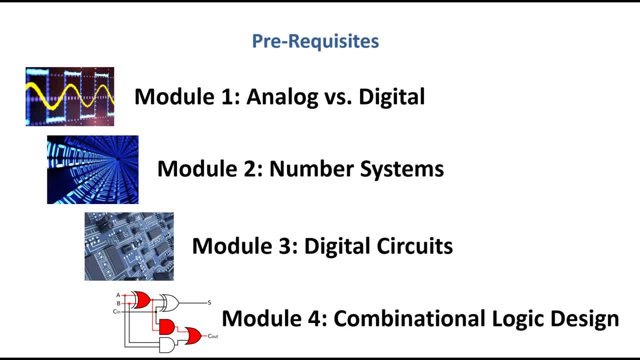 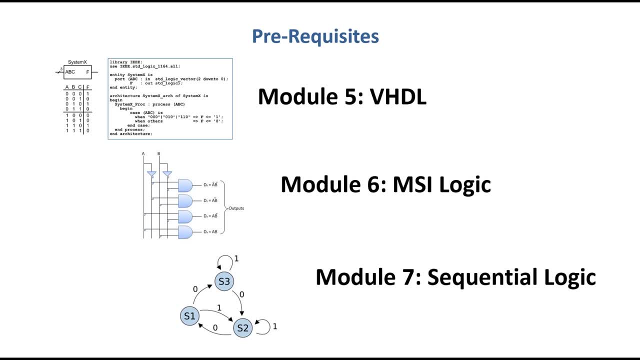 or a minimized product of sums using a carnal map, And so that was what module four was about. Then we turned our attention to the modern digital design flow and we started looking at hardware description languages And in the prior class that feeds into this class. 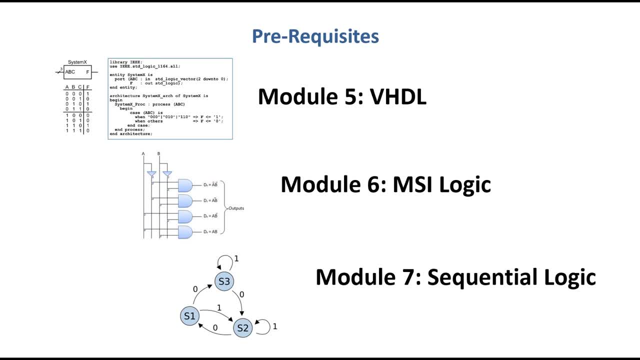 we looked at VHDL as the primary mechanism to design these digital systems. VHDL is a language and it gives us the ability to describe a logic circuit in a language, So we actually type out the functionality of the circuit, including the inputs and the outputs. 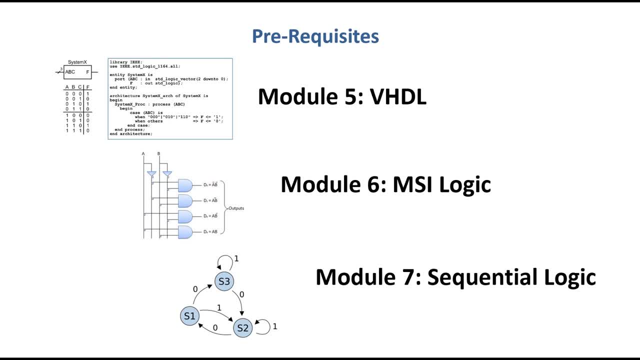 how the logic is going to operate, And it was very powerful because it gave us the ability to simulate the result and make sure that the circuit is described properly before we actually build the circuit. Then the real power of the modern digital design flow is that once you have the VHDL, that's accurate. 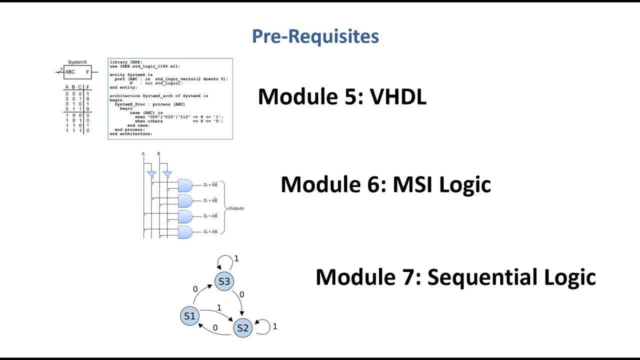 you can use an automated tool to actually synthesize the circuitry for you, And so we learned how to synthesize our VHDL and create essentially a bitstream or a netlist that can be implemented on a programmable logic device. So we used an FPGA before, in the prior class. 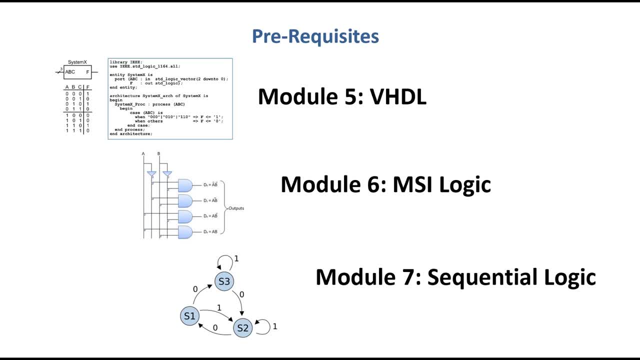 and it was very powerful because we could immediately start building very large digital systems using VHDL And we allowed the tool to create the logic for us And that allowed us to design at a higher level of abstraction. And then we moved on to MSI logic. 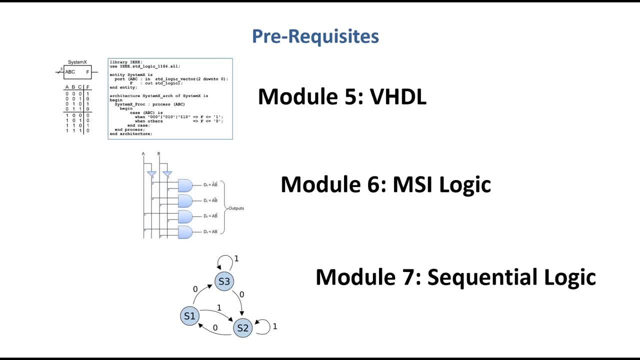 which is just looking at some basic combinational logic circuits. So things like encoders, decoders, multiplexers, And it was just to get a taste of. okay, there are combinational logic circuits that are so common there's no need for everybody to design them. 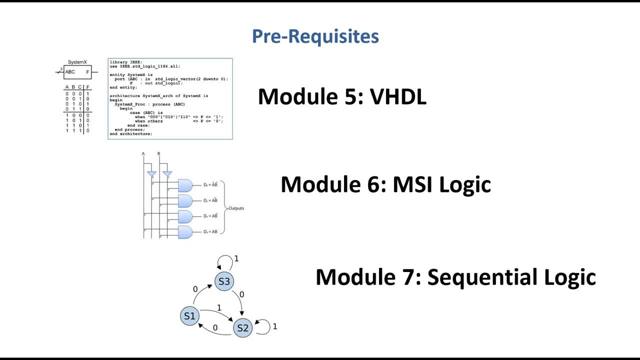 So what we'll do is we'll have them be designed for us And then we'll just purchase them or use them. And we just looked at some common ones. But, more importantly, we looked at how you could use the classical digital design approach. 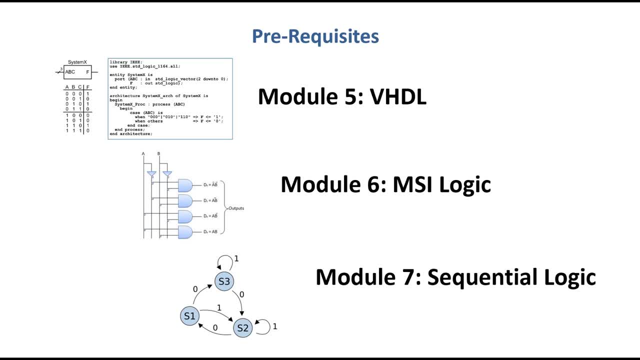 to actually build them yourself. So if somebody said, build a multiplexer, all you really need to know is how a multiplexer is supposed to work, create the true table and then synthesize the logic using a Karnaugh map, Or you could if you know how it worked. 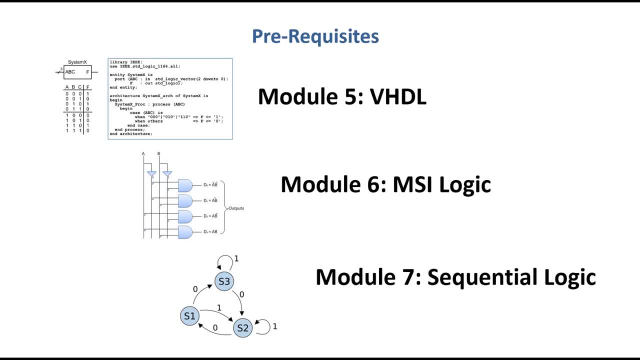 you can describe the multiplexer in VHDL and synthesize it using an automated CAD tool. Finally, we wrapped up with sequential logic. This is where we started looking at circuits that could create their outputs based upon both the current value of the inputs and also the past values. 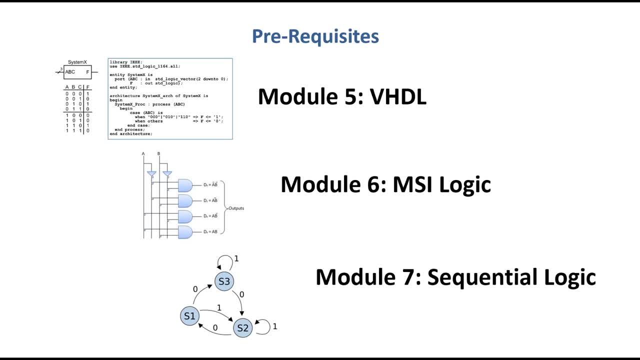 So whenever you're talking about past values of something, you're implying that you need storage. So a sequential logic is circuitry that has some sort of storage mechanism. Storage is not in this context. memory arrays, so things like DRAM in your computer. 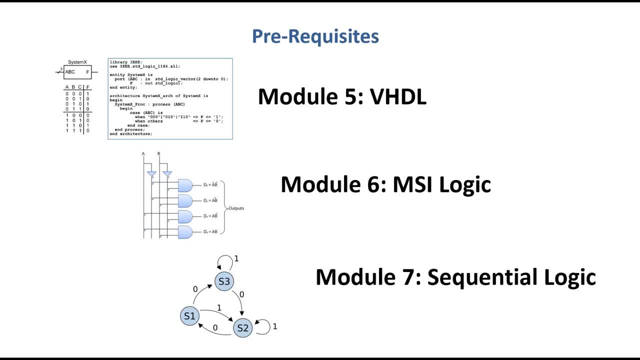 What we used was a DRA was a D flip flop. So a D flip flop was a very fast storage device that could store one bit at a time and it would only grab the input and store it upon a triggering event, And the triggering event that we used was the rising edge of a clock. 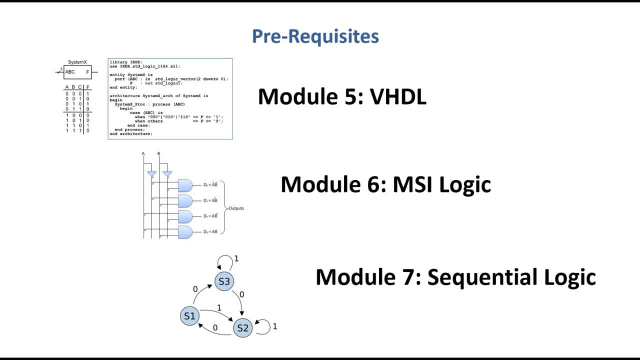 So you should have all of that knowledge in your past, or you should at least know what I'm talking about roughly- before taking this class. And so now we turn our attention to. what is this class about? What is logic design about? Well, for this course, 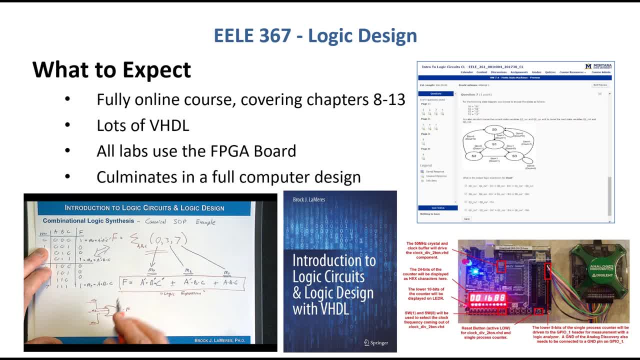 what we are going to do is we're going to continue using the same textbook And really what we're going to do is: in 261, we cover chapters one through seven. In this class, we're going to cover chapters eight through 13.. 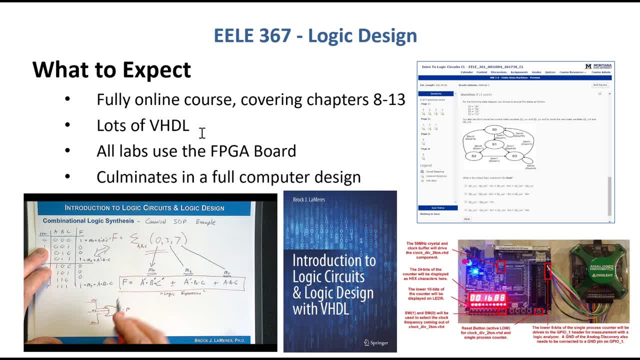 This class is heavy in VHDL, So every lab is going to be done in VHDL. Almost all of the homeworks are going to be done in VHDL. All of the labs are going to use an FPGA board and we're going to get to the point where everything will come together and we'll build a full computer system. 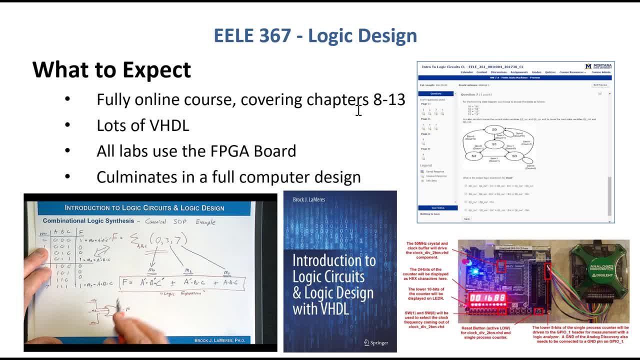 So what to expect in this course, before we get into the individual content, is it is a fully online course. OK, so you're going to be, instead of a lecture, you're going to be watching videos that I created for you. You're going to be doing homework in the form of either multiple choice quizzes within our bright space learning environment. 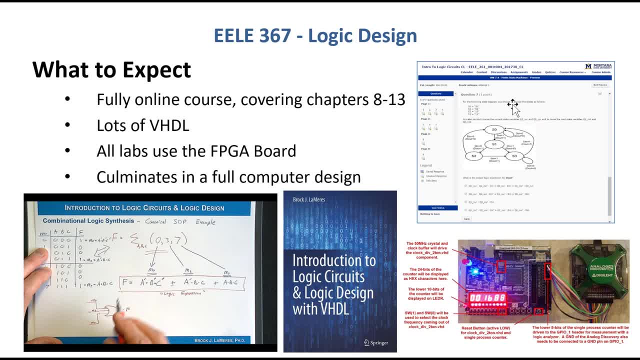 or you're going to be doing VHDL simulations and uploading screenshots. You have the textbook. of course, video and the textbook match Exactly, So you can read if you prefer that, or you can watch videos if you prefer that, or you can do both to get kind of a different perspective. 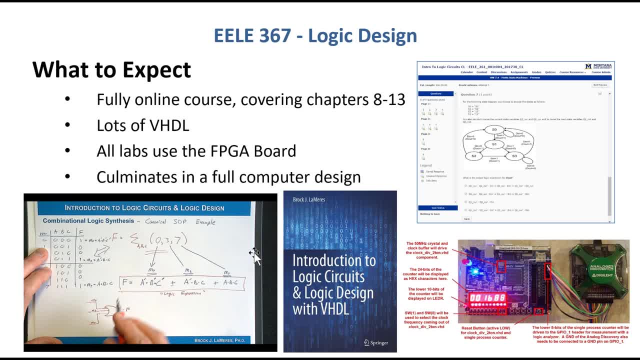 But keep in mind, I wrote the textbook and I did the videos, So it's kind of me describing the information in just two different modes for the labs. You are only going to use the VH or only going to use VHDL, and you're only going to use the FPGA and the analog discovery. 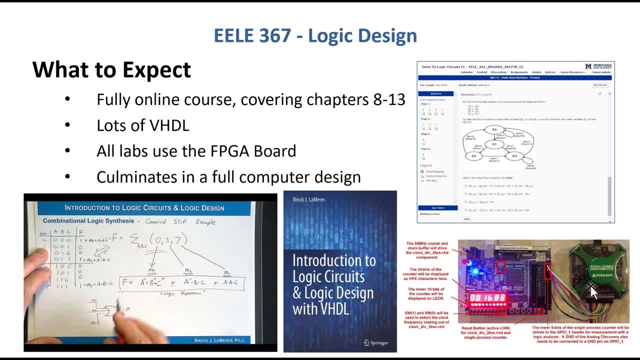 So you don't need to use any discrete parts or your breadboard. You're just going to be doing a whole ton of VHDL. So that's where we are Going. So let's take a look at the. let's take a look at the topics that we're going to cover. 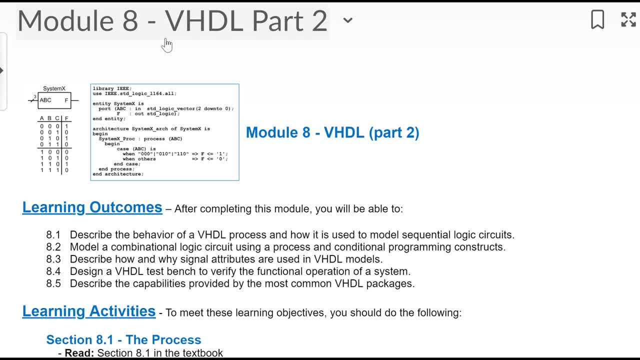 So we're covering chapters eight through 13.. What we're going to do is we're going to start off with what we call VHDL part two. So at this, coming into this, you should have been able to create a very basic combination of logic circuit using VHDL. 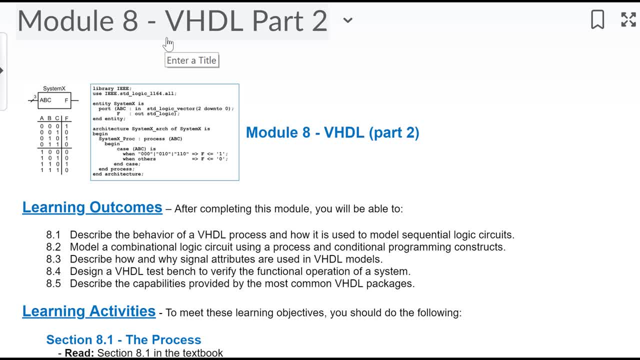 So you should understand things like what an entity is, you know what an architecture is. Do some simple signal assignments With some logical operators So you can create a three input and gate. or you can create a very simple sum of products form combination logic circuit. 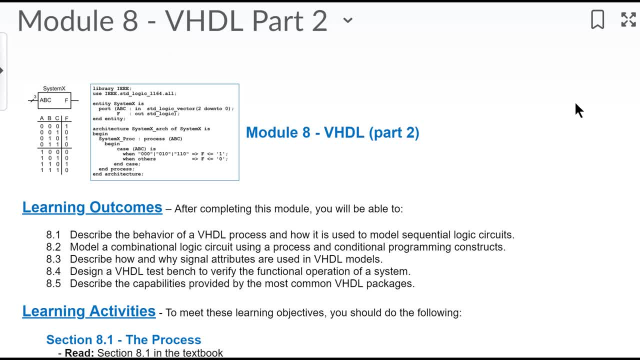 Once we get to this class, what we want to start doing is looking at the rest of the functionality of VHDL. So this is where we're going to start looking at. how do you model events that are triggered? So, instead of being continuously assigned to the output like a combination logic circuit, 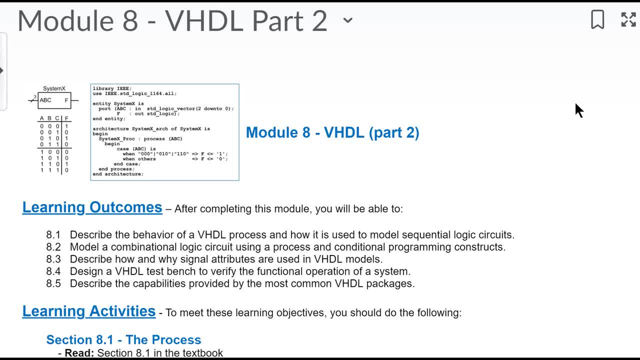 how do you create a D flip flop or how do you create a finite state machine? So we begin looking at more advanced techniques to model behavior, such as using a process, and how to trigger the process and do sequential signal assignments. So the first module we cover is just looking at the rest of the functionality within VHDL, so that you can model all of the types of digital logic circuits that we see in modern digital systems. 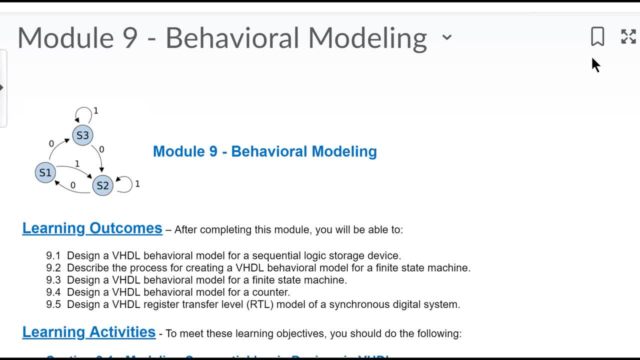 The next module is where we just get some practice doing it, So we learn all the constructs of VHDL. Then what we do is let's just start looking at the most common circuits that you have. So we look at things like building a combinational logic circuit using an if then statement or a case statement. 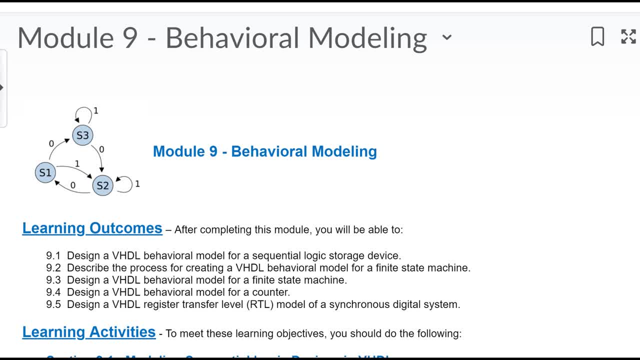 How do you create a D flip flop model? How do you create a finite state machine? How do you create a counter? How do you do register transfer level? So we look at the most common things that you need to design in digital logic and we just do examples of it. 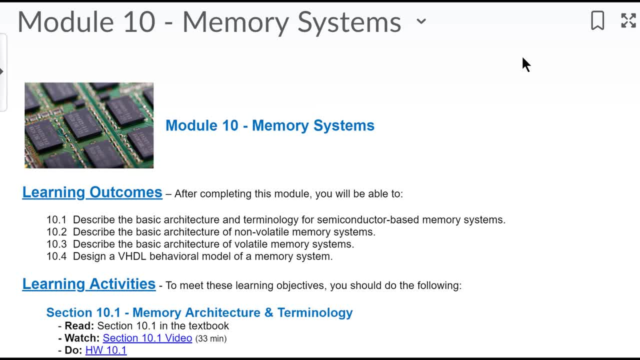 Then what we do is we turn our attention to memory systems. So if you're going to build a computer someday, you need a large array of storage. That's not a D flip flop. OK, so with D flip flop is something we store information for. 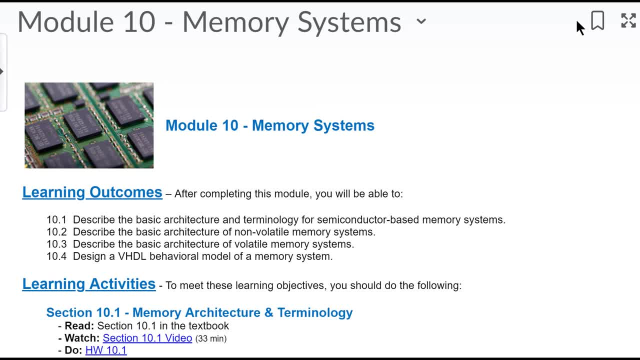 like a register or or A finite state machine, But memory systems are different. Memory systems are where you have gigabytes of information that is stored in a different technology. So we need to. since we're going to have that logic functionality, we need to know how to model it in VHDL. 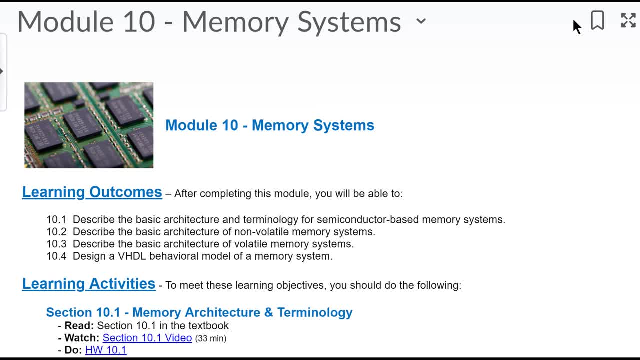 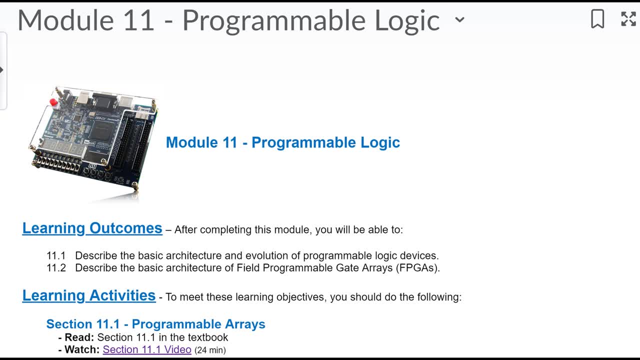 So we look at some common technologies used to implement semiconductor memory systems, Then we look at the VHDL to model in. Then we get into programmable logic, just a short module that just looks at the common technologies that we use to implement some of these digital systems. 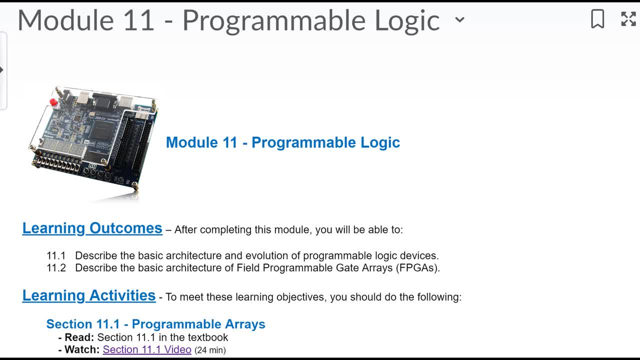 When we're prototyping, and sometimes just the final product. But we we cover programmable logic because that's what we use in the lab. So we finally get to the point where we know enough about what we're trying to model that we're ready to look inside of the FPGA and figure out what they actually put on there. 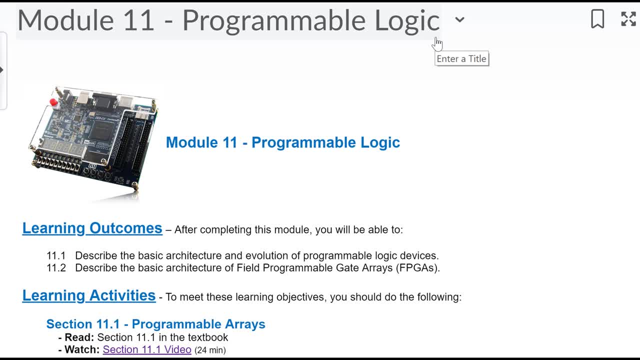 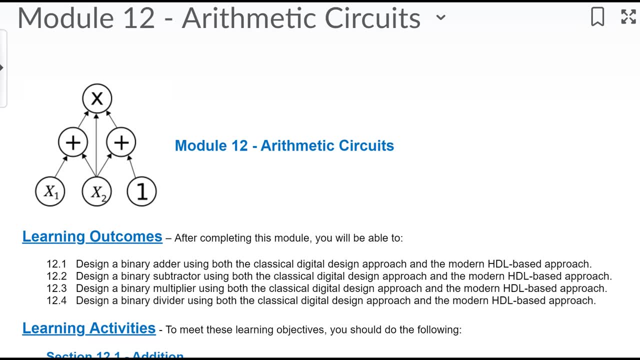 So once we look at this module, it's kind of neat because you actually, as you look at all the programmable little blocks inside of it, you'll understand what they do and how to actually build them. So then we finally wrap it up with looking at arithmetic circuits. 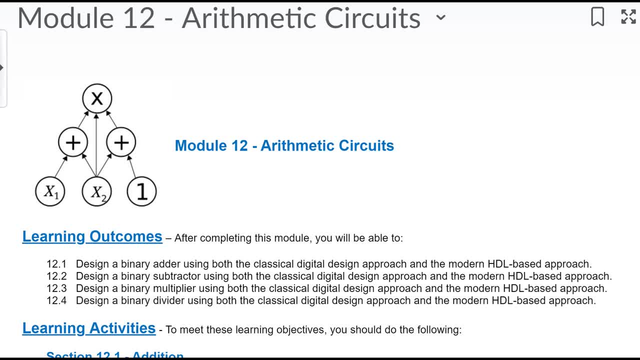 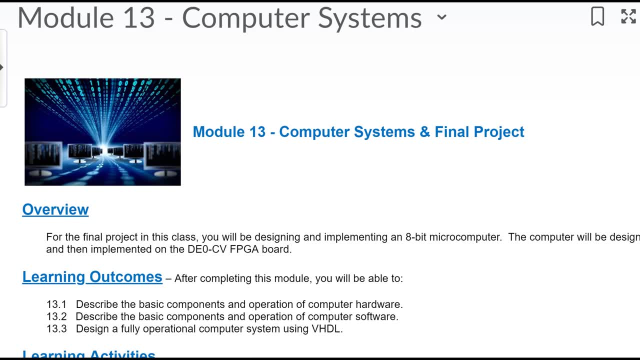 And this is going to be More complex- circuits, so things like adders and subtractors and multipliers and divides, And once we get through module 12, you get to the end and you will realize that you have put together all of the information needed in order to build a computer system. 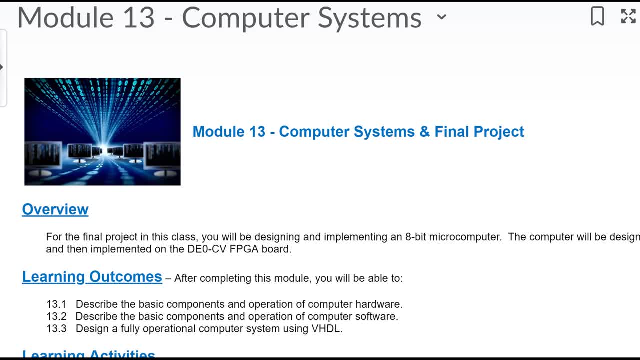 So you're going to be able to build the CPU of a computer system, the registers, the data routing in between it, the finance state machine that controls the execution of instructions. You're going to be able to build the memory system that can store, read only memory or read only information. 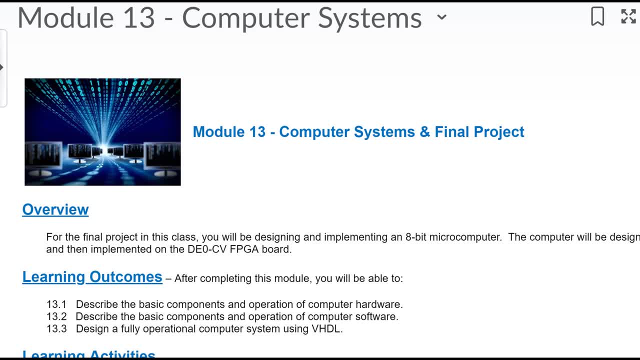 You're going to be able to model the memory that stores volatile memory, So things like read, write memory. you're going to be able to model output registers And we look at all of these different things that we've covered and you put them all together in the most common digital logic system that there is. 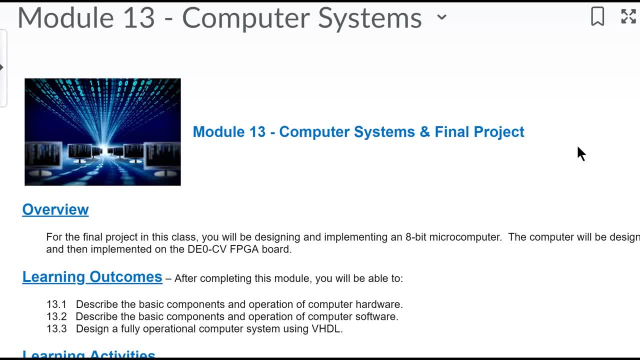 which is a computer. So this course culminates with actually designing a complete eight bit computer that is in VHDL. You're going to simulate it using a simulator, You're going to synthesize it using a automated CAD tool And you're going to put the whole thing on an FPGA and run programs. 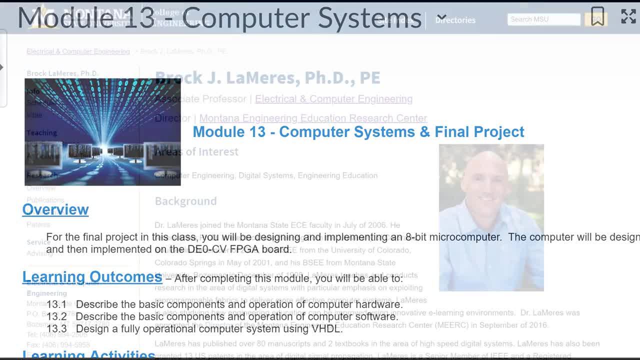 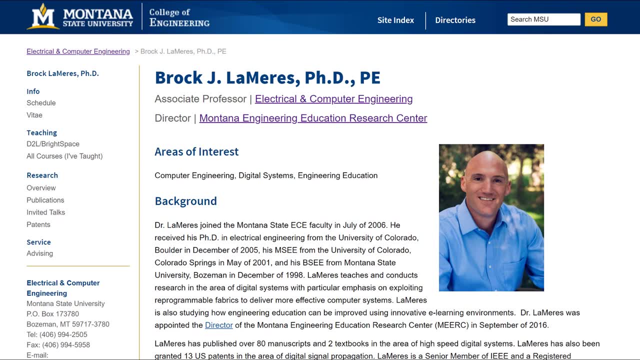 So it's going to be kind of a culmination of the entire course. Before we get to the course logistics, let me give you a very brief background on myself, just because I'm going to be the person that you hear and see in the videos. 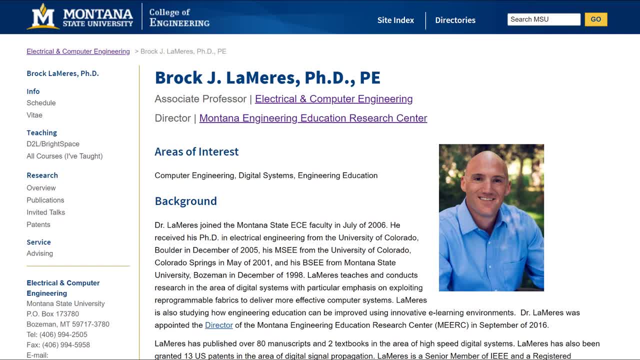 And also I'm the person that wrote the textbook, So and also I'm teaching the course, So sometimes it's good to know who is at the other end of this class. So again, my name is Brock Lemire. You can call me Brock. I've been a. 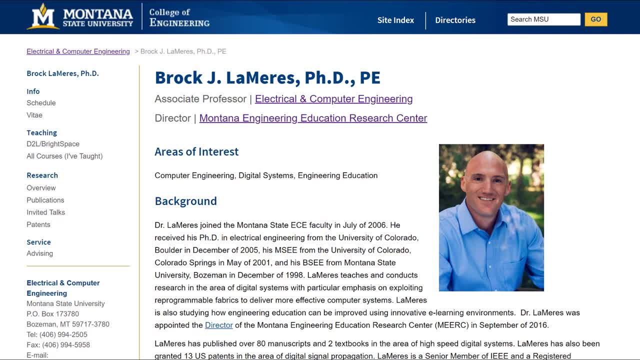 Professor at Montana State University for 12 years now. I got my bachelor's degree from MSU back in 98.. I then went to work as a hardware design engineer for Hewlett Packard in Colorado, And what I did there was I designed basically digital systems. 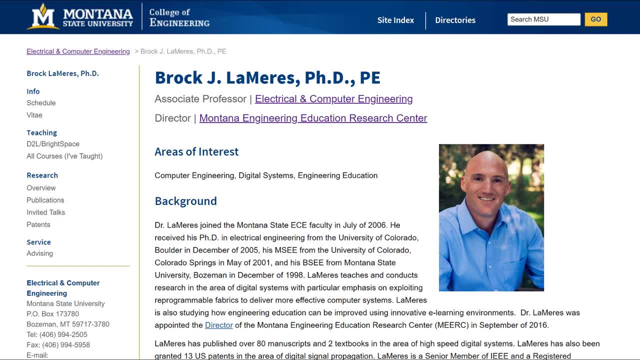 They were acquisition systems for electronic test equipment, So logic analyzers, And so what I did was a lot of FPGA design work, a lot of print circuit board design, a lot of just digital logic design. So I did this in my past life. 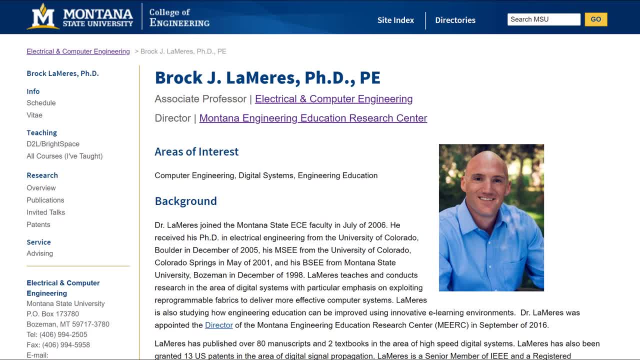 And I worked for Hewlett Packard for eight years while I chipped away at getting my master's and my PhD at the University of Colorado. So I got my PhD from the University of Colorado in 2005.. And I ended up coming back to Montana State in 2006 and joined the faculty in the electrical and computer engineering department. 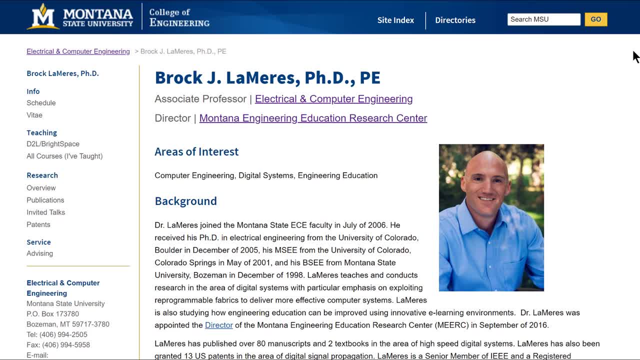 So, since coming back, what I've mainly focused my research interests in, or my research area has been on, digital systems. So you know, digital systems, So digital systems, are an essential part of my life. So I've done more of the digital life side of things, in terms of how I do stuff, And I've also done more of the engineering and the engineering in terms of how I play with it. 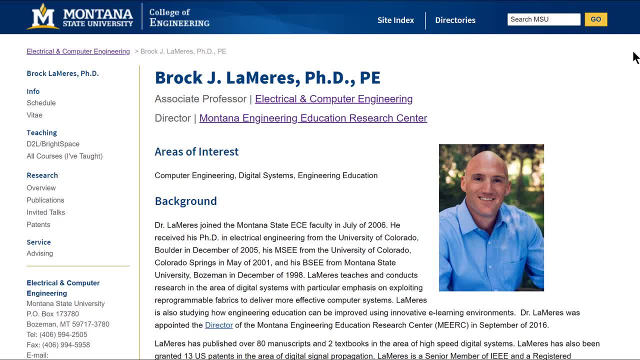 I've also done some of the programming and the programming that I do with the software abilities. I've also done some of the programming and the programming that I do with the software abilities. you know, digital systems are everywhere, But what I've been doing technically is I've been 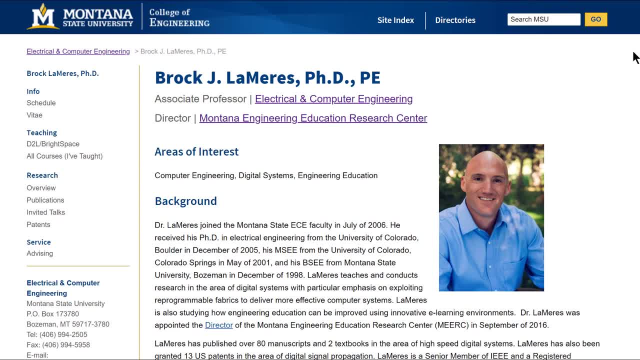 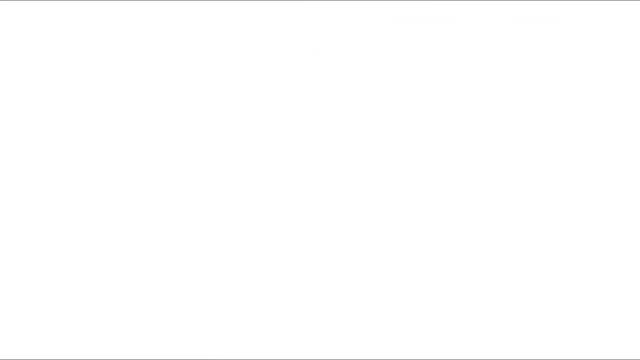 looking at creating reconfigurable computing systems, all FPGA based, to optimize the computer for a particular application. And what I've been doing is I've been doing a lot of work for NASA recently, where I've been building these space computers for various applications, And this 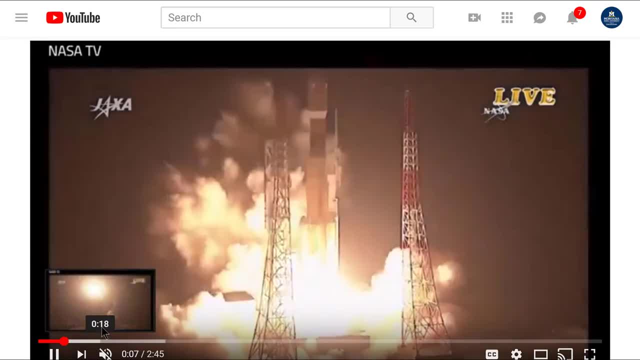 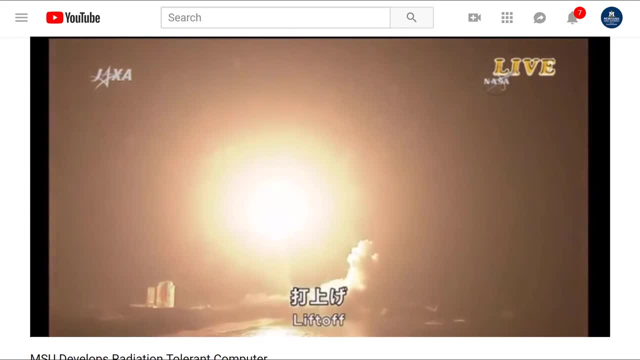 has allowed me to kind of. this has allowed me to kind of stay up to tune or up to date with what is actually being used in the real world, And also we've been doing some exciting things where students that work for me have been able to build, you know, real, real hardware. that has been 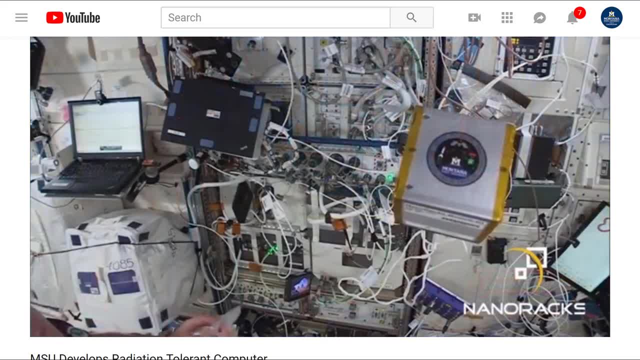 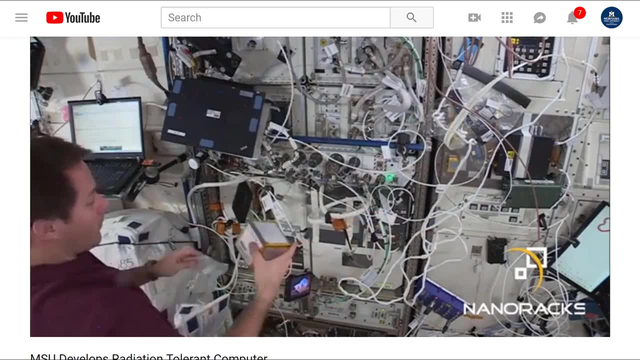 flown in space. So we have a computer right now, as I speak, that's on the International Space Station getting ready to be put into orbit. We just had a computer that was up there for a year where we tested how well it performed under bombardment. 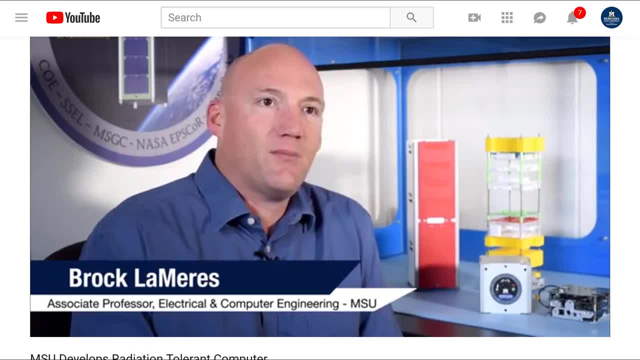 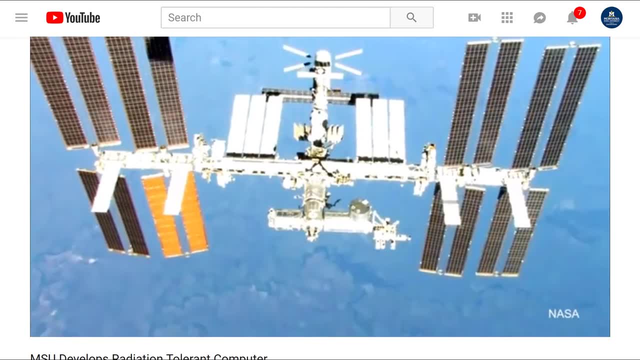 By radiation. So this is the type of stuff that I do for my research. I also am in the director of the Montana Engineering Education Research Center And what we do there is we look at how can we improve engineering education. So you know it's engineering education is. it's a difficult thing. 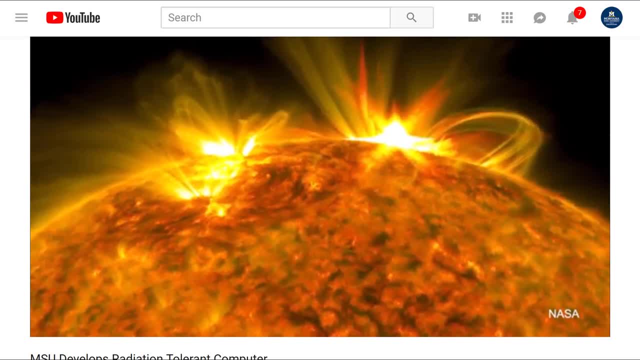 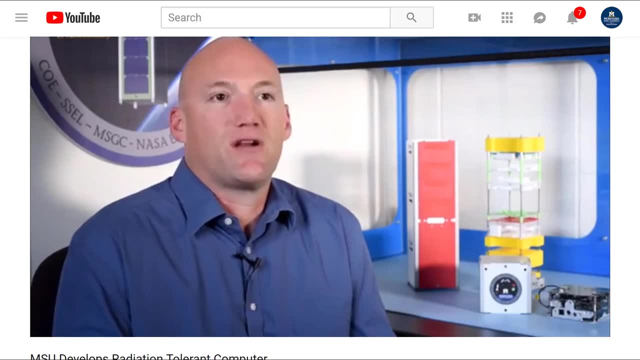 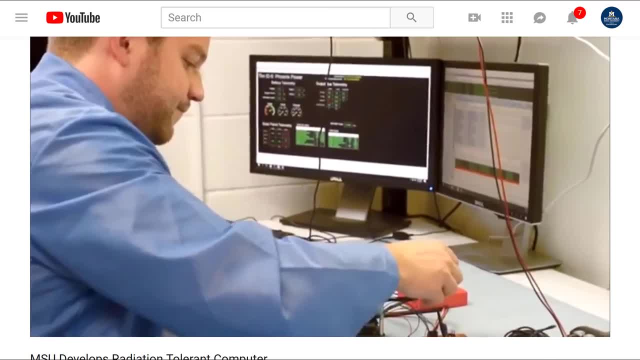 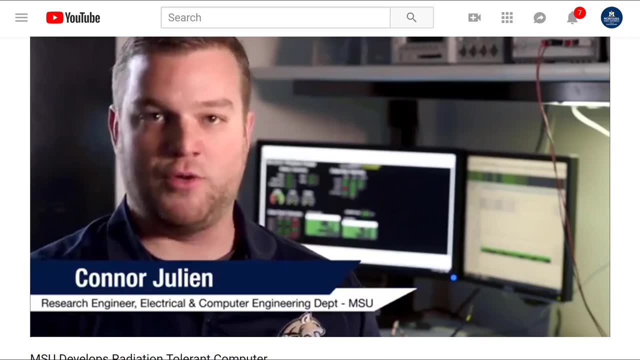 it's not trivial and it's becoming more and more complex because there's just so much more information available. The systems that we build are so complex that we just need to think about new ways to try to educate people. So I've been the director of that for three years now, And 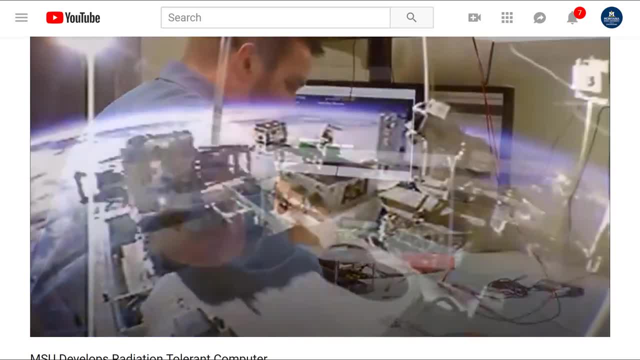 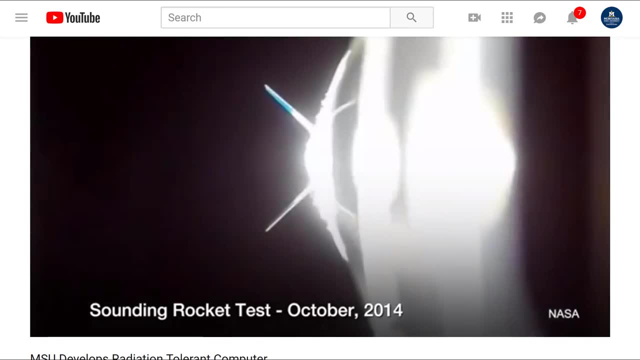 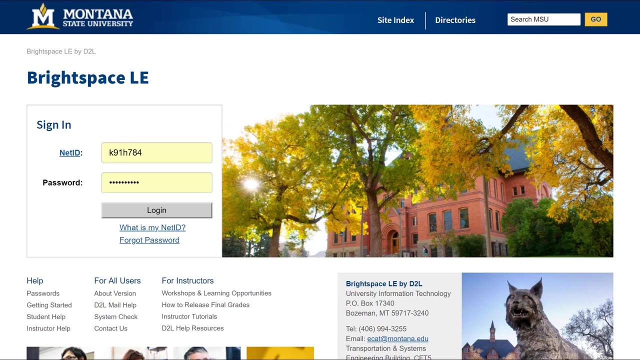 I've received numerous grants from the National Science Foundation to kind of conduct studies on how to improve engineering education, And I do a lot of it with MSU students. So that is me. now Let's take a look at the course logistics So you can actually get started on the class. Okay. 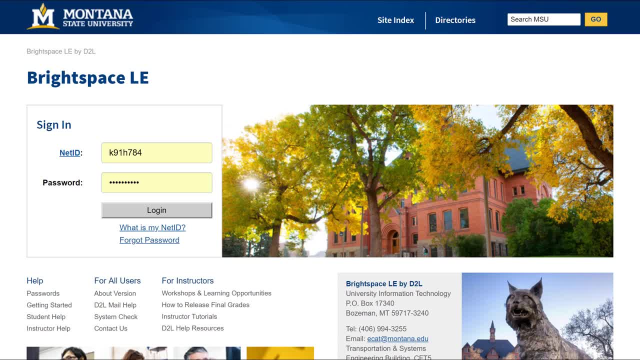 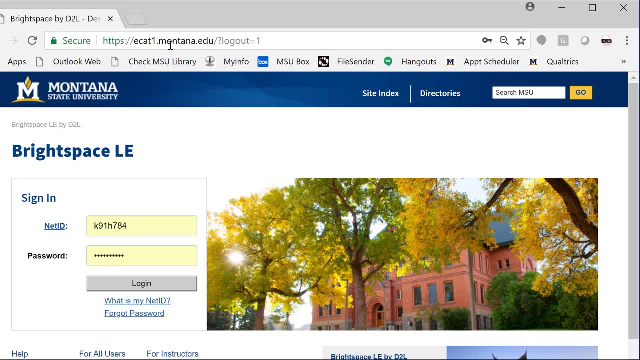 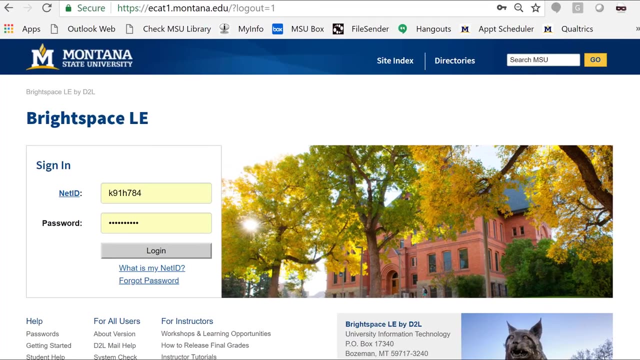 so this online class is going to be administered through our bright space learning environment. Okay, so the address for this is ecatmontanaedu And it'll redirect you a little bit to this ecat one, But anyway, just ecatmontanaedu, And you log into this using your net ID and password. 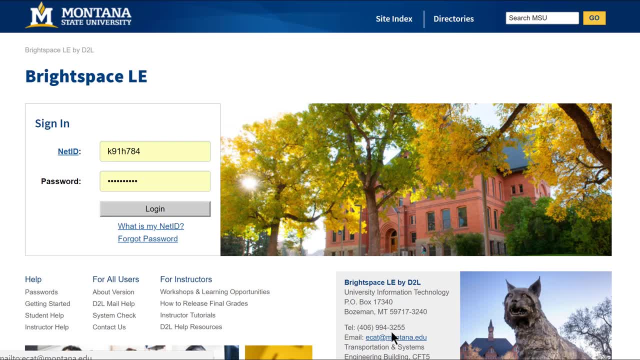 And once you do that, if you have any problems with logging in, you're going to want to call this 994-3255 number and they'll help you get in there. Once you log in, what you're going to see is all of your active courses And mine is going to look. 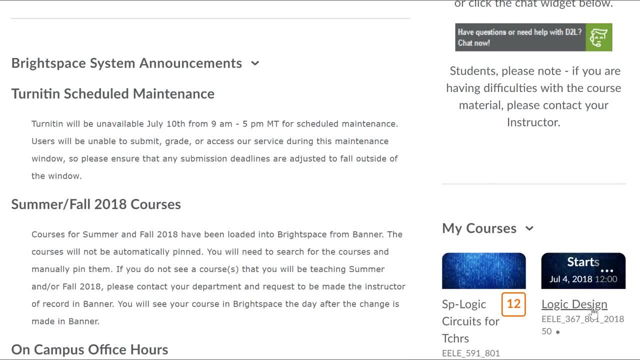 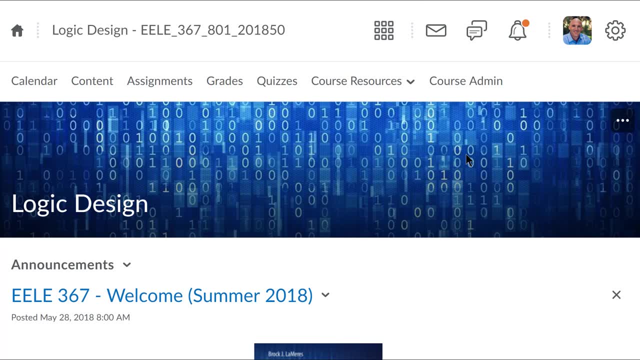 a tiny bit different than yours because I'm the instructor, But I've got my course down here. I'm going to come down to logic design And this is what you'll see when you enter the course. So I have, you'll see, this banner and it says: logic design lets you know you're in the right. 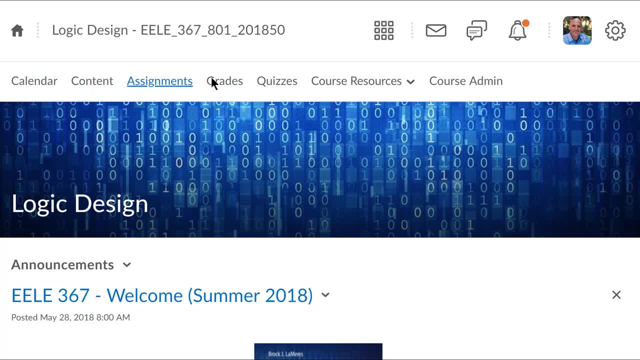 place Along the top of bright space. you're going to see all these different tools, But what I've done with this course is I've linked everything- Content, So you really should only ever have to go into content if you want to find access to. 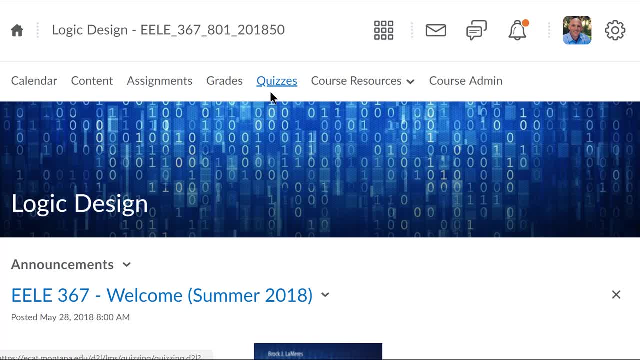 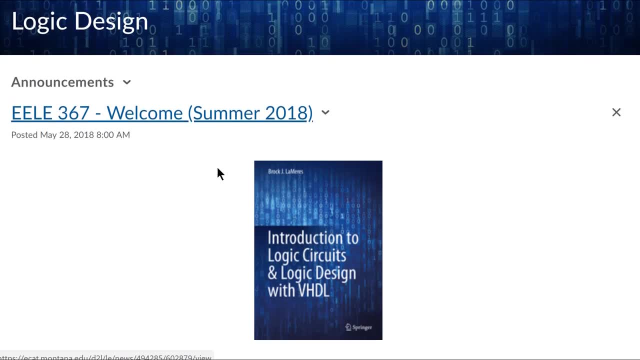 everything. So I've linked all the assignments and quizzes and stuff like that, But content is where you find the content. Okay, So when you come in here, I put an announcement that just says welcome, just as a landing pad. So you know you're in the right course. So this is where you come. Now look. 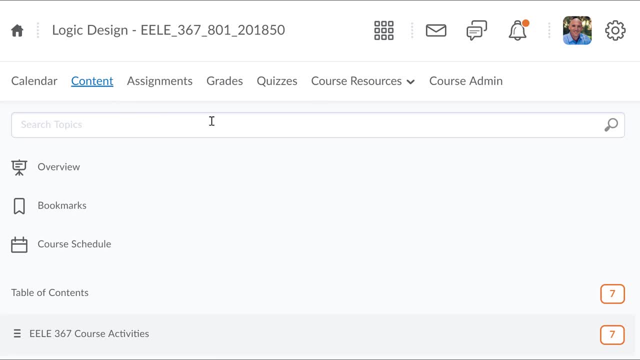 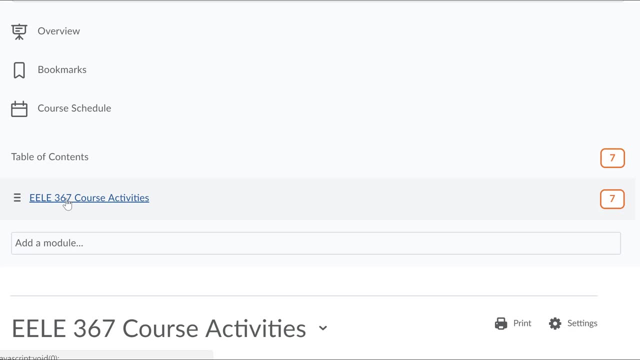 at. let's go to content right now and take a look at the course. Okay, So when I come into here, what I'm going to see is I'm going to see this one folder called ELE 367- course activities. Okay, So if I click on that, what I'm going to see is I'm 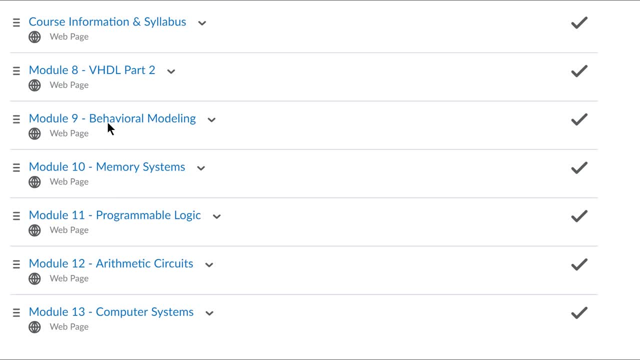 going to come down here and I see all of these different activities we're going to do. Notice that there's a page for every module. Okay, So you're going to see module eight, VHDL. part two On these pages is the links to everything. Okay, So this is the links to the reading assignments. 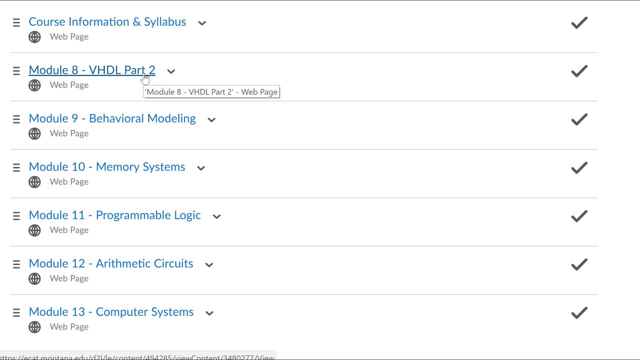 what you're going to be doing, the videos, the homework, where to upload your homework, where to take the quizzes, et cetera, et cetera. Okay, Click on these and just work all your way through them. If I start off with course information and 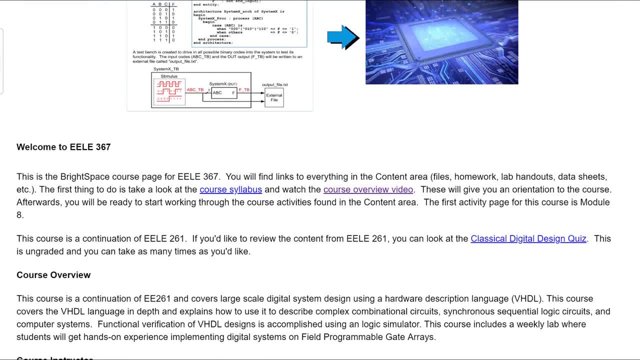 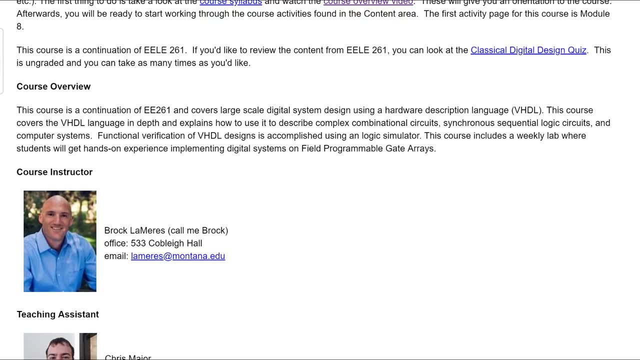 syllabus. what you're going to see here is just a brief overview of the course. that is the stuff in the in the syllabus. But this is where you would find links to, to stuff like my email. So when you come in here you're going to see the course syllabus. You obviously have found the course. 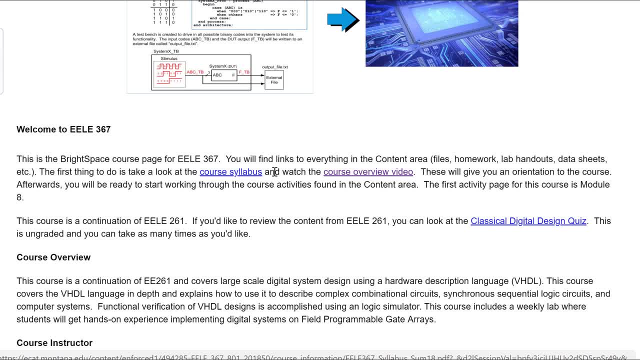 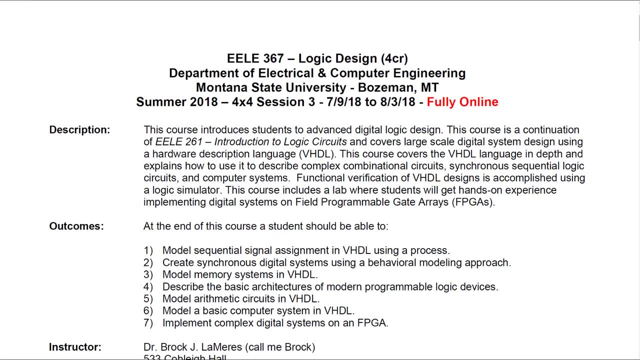 overview video. But let's take a look at the course syllabus first before we start flipping through the pages of the course. All right, So here's the course syllabus And you know description of the course. So we already kind of covered that This is the part two of a course. 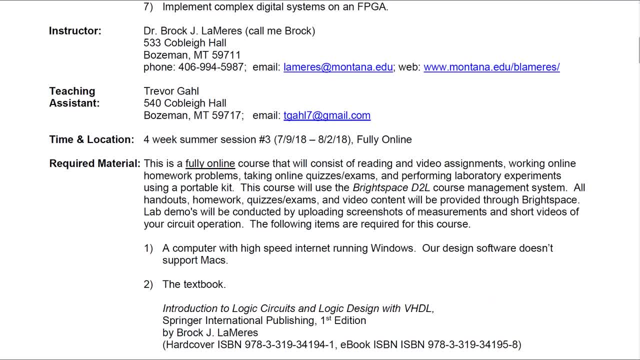 Outcomes You already. we already covered that. You already know me. Here's the link to my email, But we also have a teaching assistant for this, So you know this is an accelerated class, So you're going to want to have. 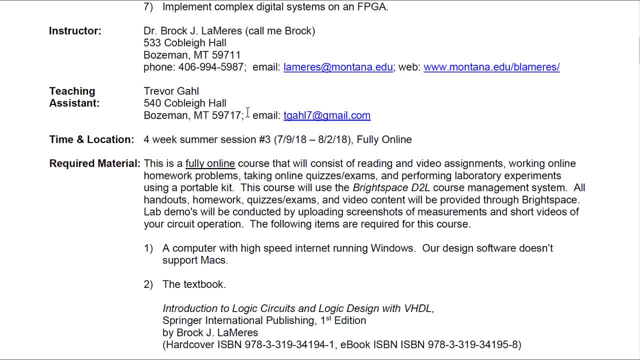 rapid feedback. So we actually have a, a Trevor Gall, who is going to be helping out this summer, And his email is right here at TGall7 at gmailcom. So when you email for help, you should always email both of us. 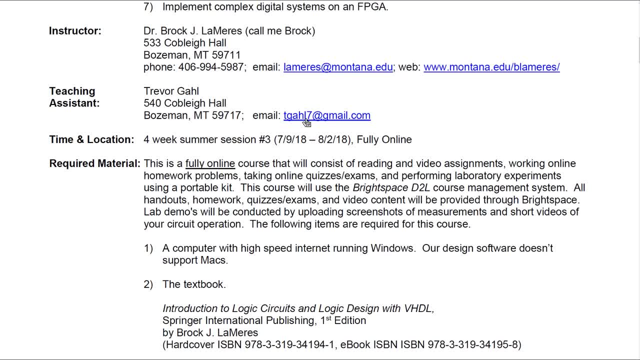 And the first one. one of us will reply as soon as we can. okay, all right, here's the big one. this is a four-week summer session course. now, this is an accelerated format and the whole a semester-based course, is going to be done in four weeks, so you're essentially every day of that you engage in. 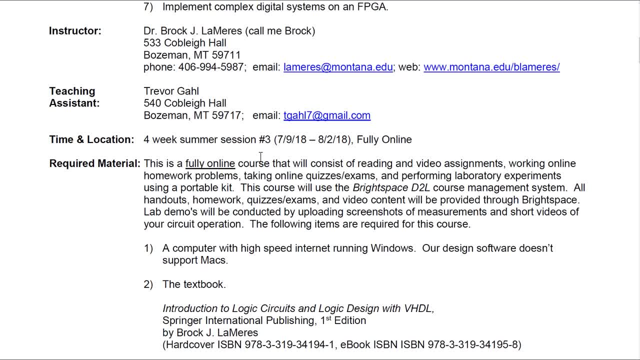 the course is like a whole week's worth of learning. now that is critical, because it's important that you know that this is an accelerated course. this is not a short course. this is a full semester-based course that we're going to do in four weeks. that means it's going to be nearly 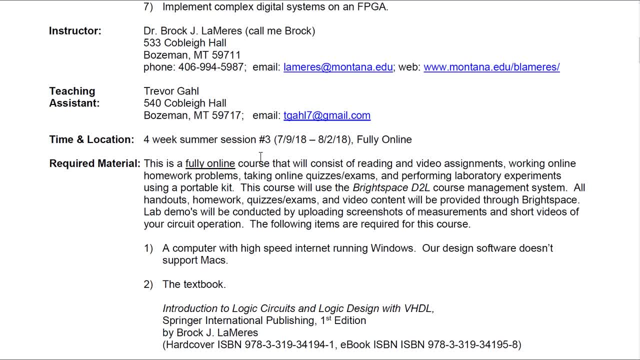 impossible if you're trying to work a full time job, or it's going to be impossible if you're trying going to take a week off during it, because that would be like missing a month of school during the spring semester. so you got to make sure that this is, if you take this course, this is your. 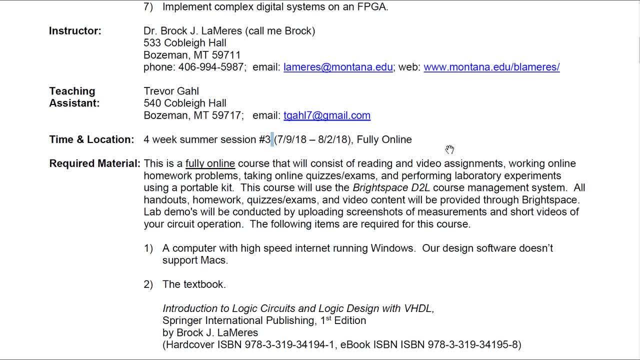 number one priority and be prepared of how much time it's going to take. the good time. the good thing is it's over in four weeks and it also is fully online. so that means you don't have to be on the msu campus to take this course. everything can be done remotely. it's the course is designed. 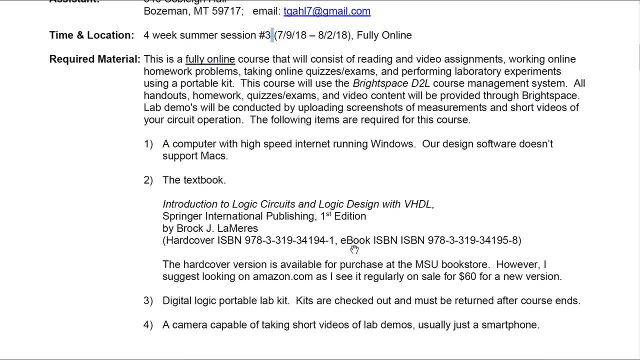 so you can do this from anywhere in the planet, as long as you have the following four things: you need a computer with internet connection running windows. now, that's critical. we- the software we're going to use- does not run on a mac. okay, so you got to have a windows machine. you can do it with a linux machine, but i'm assuming 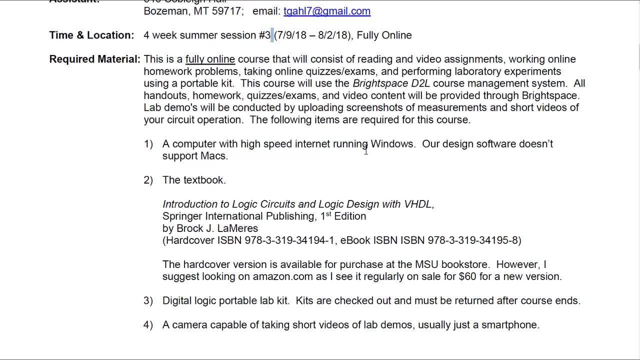 everybody has windows. you can't do it with the mac, just flat out. we the software we use, called cortis, that has the model sim simulation software and the synthesis tools. it doesn't run on a mac so there's no way to do this course without it. you have to have access to a windows. 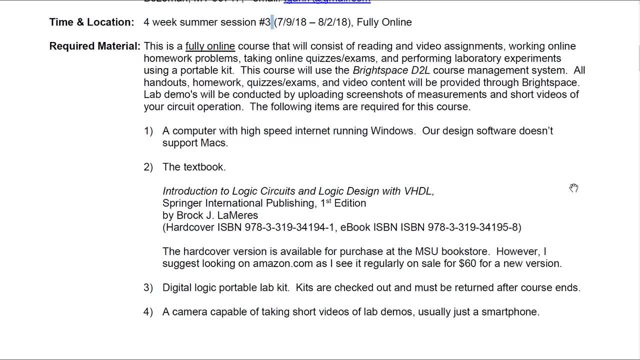 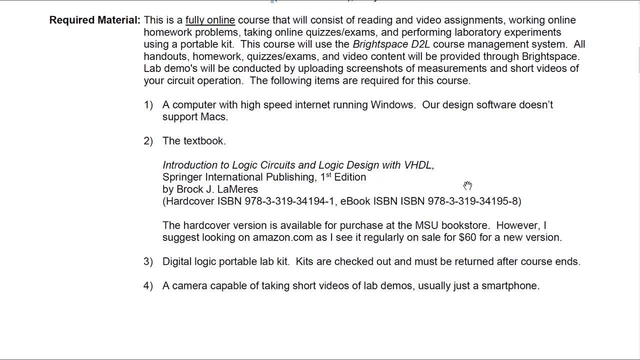 the second thing you need is the textbook. so this is the same textbook from 261 written by me. introduction to logic circus with logic design or analogic design with vhdl. and amazon usually has the cheapest hardcover version, so i usually see them for about 60. 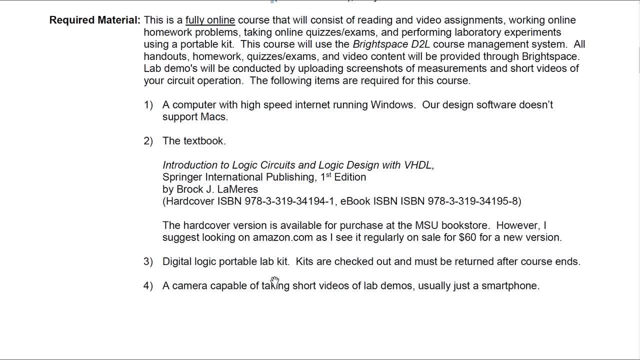 brand new. you need to have the portable logic digital logic portable lab kit, the lab kit. if you took 261 and you still have the kit, you just keep it and continue into this course. the kit has the analog discovery portable instrument that you'll see. it also has a bunch of discrete components. 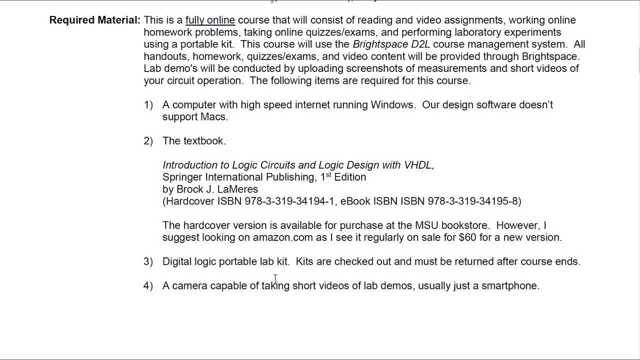 and a breadboard. in this class, we're only going to use the fpga board and the analog discovery. so if you're, if you're taking this class and you didn't just take 261 this summer, i'll ship you a kit, and so i'll be i have. by the time you read this video, i will already have sent it to you. 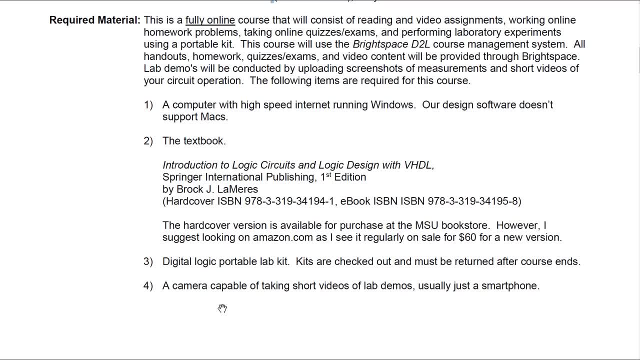 okay, and then you need a camera capable of taking short videos. the way we're going to do lab demos is you're going to actually take videos of them and upload them to brightspace. you're going to need a little camera that'll do that. almost always it's just a cell phone or a 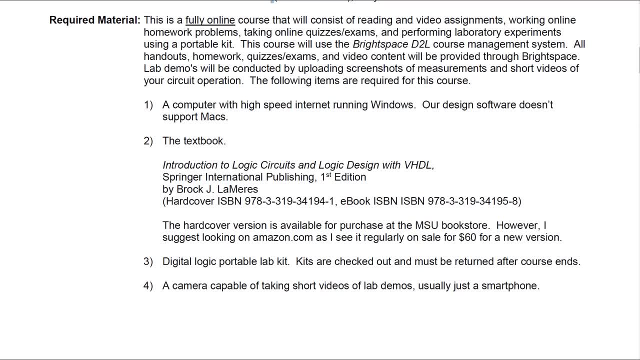 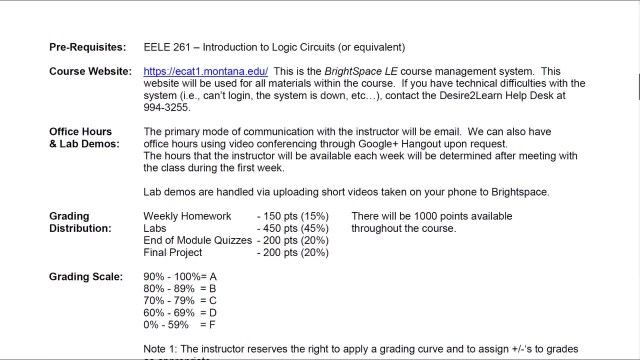 smartphone, okay, and then we're going to be doing screenshots of like measurements and so, but the main way that you're going to demo is to take a short video. okay, all right, so then, as we go through the syllabus: uh, prerequisite: you have to have had this 200 level introduction to logic. 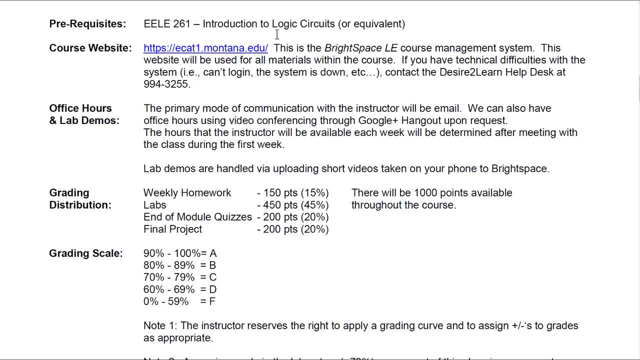 circuits class. you need to have already designed a combination of logic circuit using a k-map. you need to know what a sum of products is. you need to know what a finite state machine is and know how to use things that are already in the course as well. so, while my assignment looks like this, 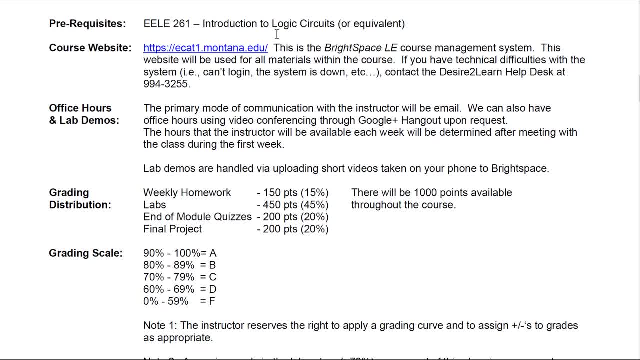 you need to know how to use all of this. it's just an example of some of the tools we've talked about, and i'm going to be using the k-map and i'm going to be using the k-map itself and, of course, if you do not have a k-map, you're not going to be able to use it for any other application, but you're. 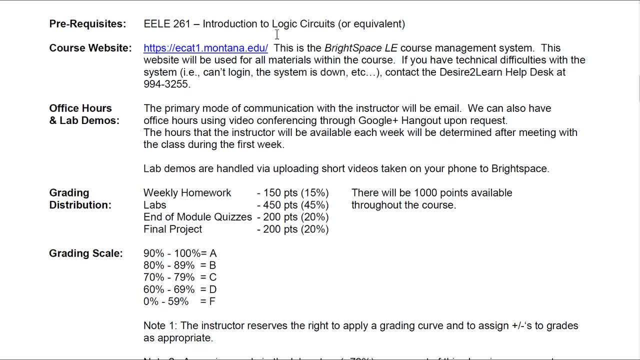 going to need to have it for module one, for the k-map, because that's obviously a very important as well as the tools that are going to be involved in this course. now, the main thing is that you uh need a laboratory type of language, but you also need to have experience, or a little bit of. 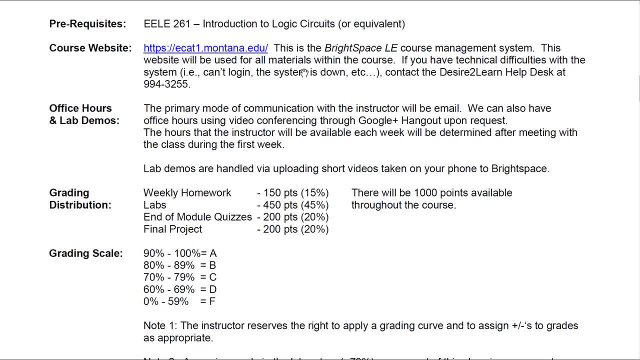 experience with vhdl or a hardware description language. if you took a class that used the another course website, I already showed you how to log in Again. if you have any difficulties with your password, just call 994-3255.. In terms of office hours and lab demos, we really don't have any. 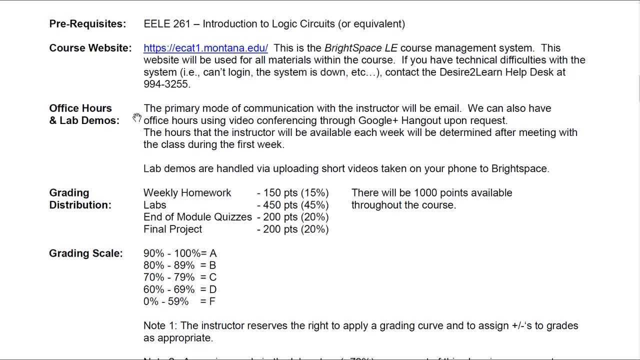 because we're always on. So the primary mode of communication for this class is email. If you get stuck on anything, email me and Trevor and we'll reply as soon as we can. I would say guaranteed within 24 hours, but realistically we're going to reply within a couple hours, Assuming that you. 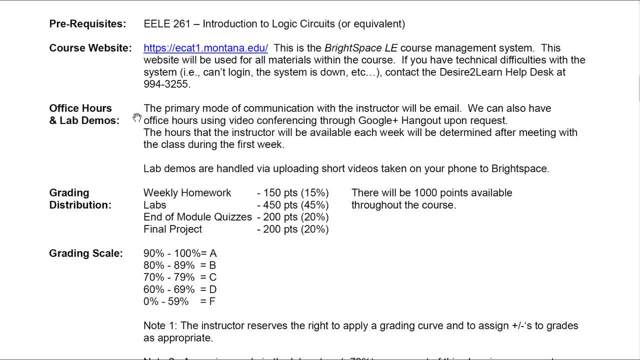 don't email in the middle of the night, okay, so we're not going to be replying at 2 am if you're working during that, but during normal hours we'll get back to you really quickly, Okay, the grading. 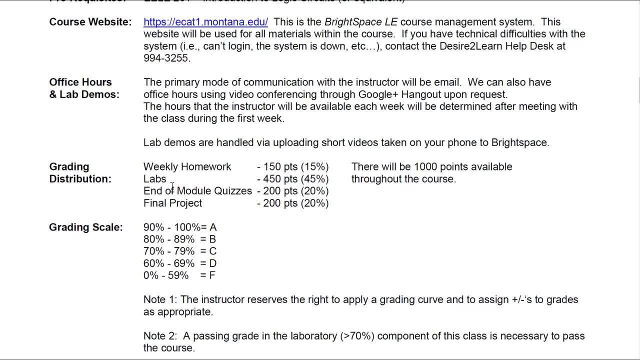 distribution for the class is: there's going to be homework, labs, end of module quizzes and a final project. The homework is worth 150 points, or 15% of the grade, And when you go in and look at your grades you're going to see that there's a thousand points available. So the homework is going to be. 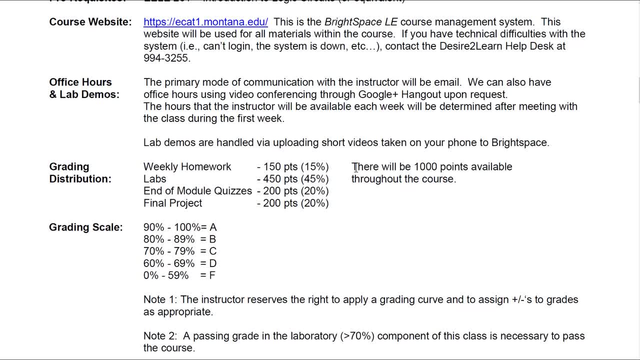 primarily VHDL simulation using model sim, but there's also going to be some multiple choice format questions. The labs are with 45% of your score. That's because the labs is where all the learning comes from. Every module is going to have an end of module quiz. 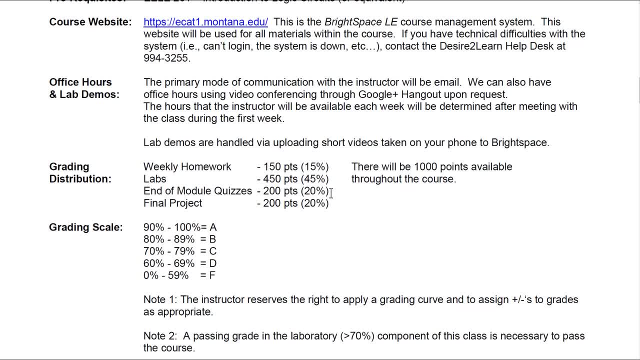 which is a multiple choice format quiz which kind of summarizes what you just learned. So there's going to be, you know, module 8,, 9,, 10,, 11,, 12.. So there's five end of module quizzes And then you. 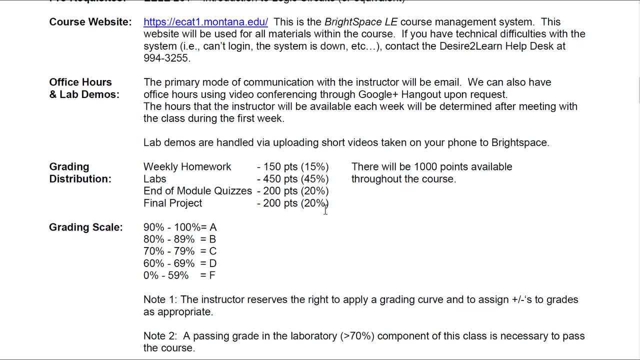 have a final project. The final project is going to be to design and implement a full computer system in VHDL and put it on the computer. So that's going to be the final project. And then you have a final project on the FPGA. If you think about it, you've got: 20% is a computer, 45% is the labs. 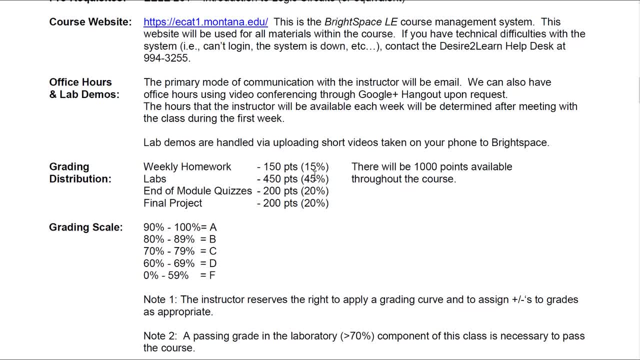 65% of this class is just VHDL. So you are going to be building large digital systems using a hardware description language and implementing them. So that's where the vast majority of the learning comes from: is actually building these systems. Of the homework, over half of it is VHDL. 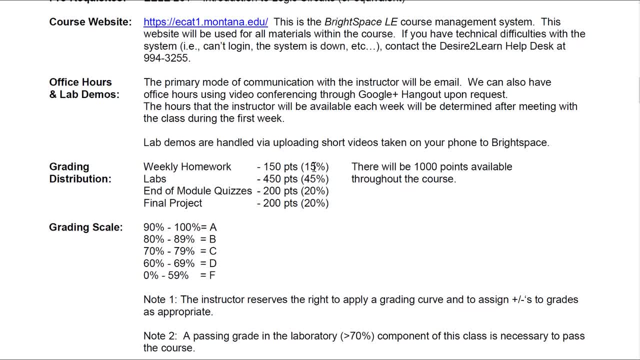 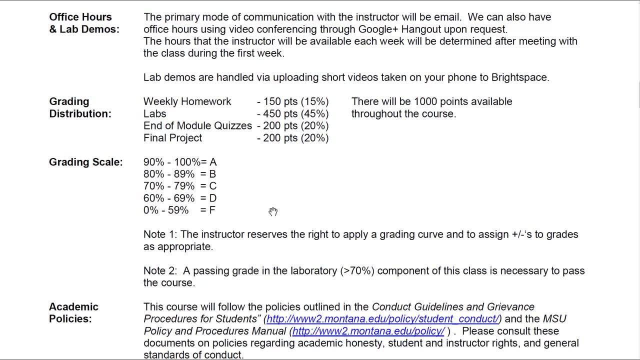 So you're talking about. like three quarters of this class is VHDL, So be prepared to do some typing. All right, Grading: I usually just grade straight. Ninety percent is an A, 80 is a B, 70 is a C. I usually don't get pluses and minuses unless it's extraordinary. 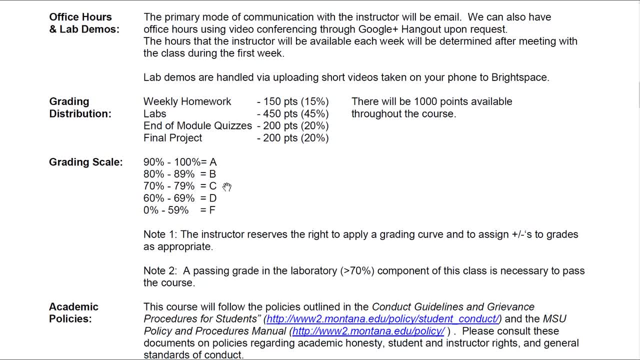 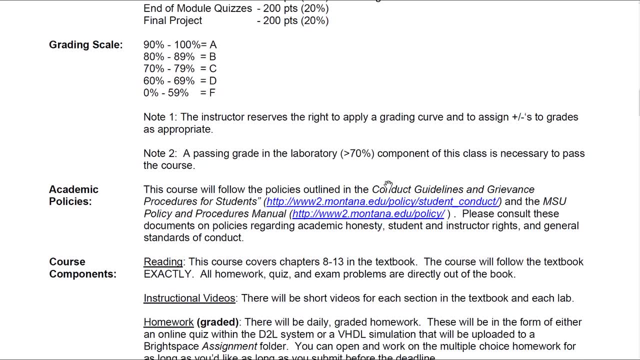 circumstances. You're guaranteed, though, if you get a 90.0001%, you will get an A. Okay, Don't worry about an A minus. Okay, But you have to pass the lab. Okay, You got to get at least a 70%. 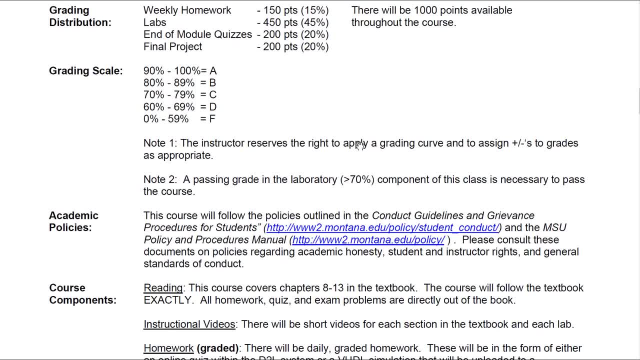 in the lab in order to pass the class. Okay, That's because all the learning takes place in the lab. You can't just plunk through the multiple choice homework problems and guess and get those right and pass the class. All the learning takes place when you build these circuits. Okay, 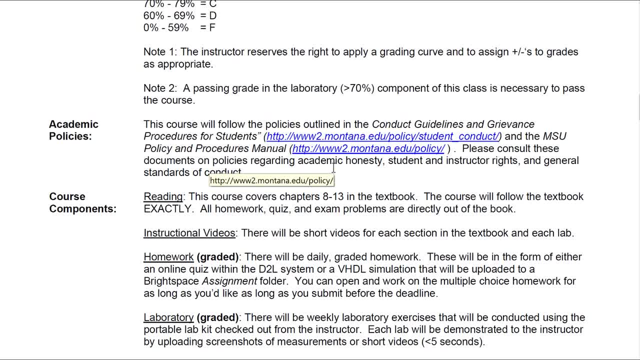 Academic policies. You can work with other classmates if you want. You just have to make sure that you turn in your own work. Everybody turns in work, Okay. So even if you're partnered up with somebody and you only have one set of files to turn in for the lab, that's fine, Just. 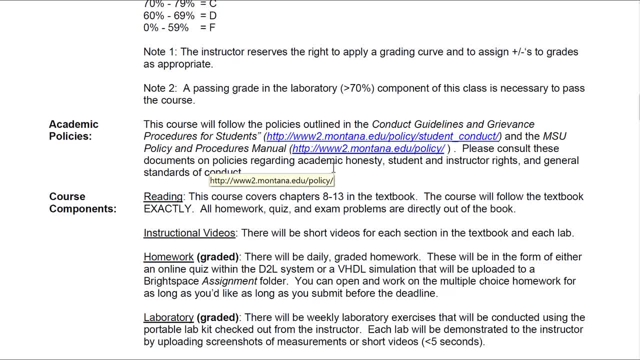 make sure to upload it to your own Dropbox so we can grade it. What the academic policy is about is: don't turn in somebody else's work that you didn't do. Okay. So there's a big difference between working with somebody where you're both collaborating at one. 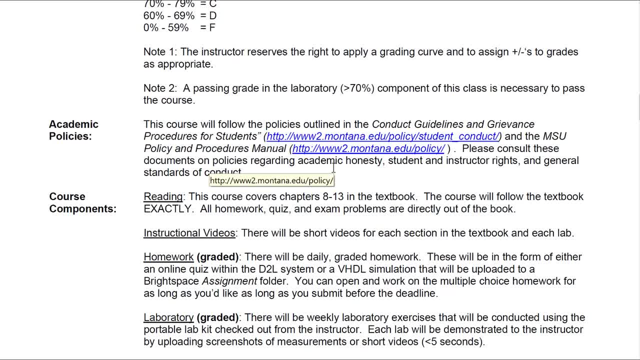 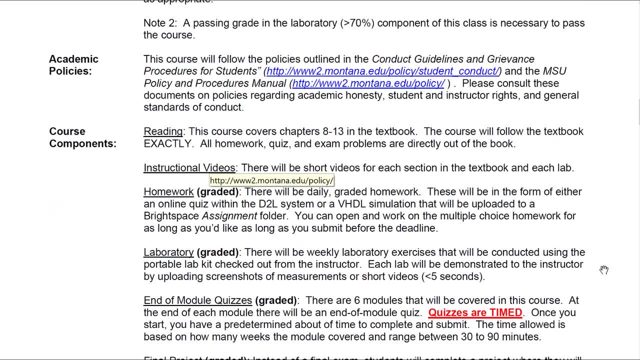 computer and you generate one design file, versus somebody did the problem for you and gave you the design file and you uploaded it. Okay, So it's common sense: Don't cheat All right Course components. How are you going to learn all this stuff? Number one: we have reading assignments. 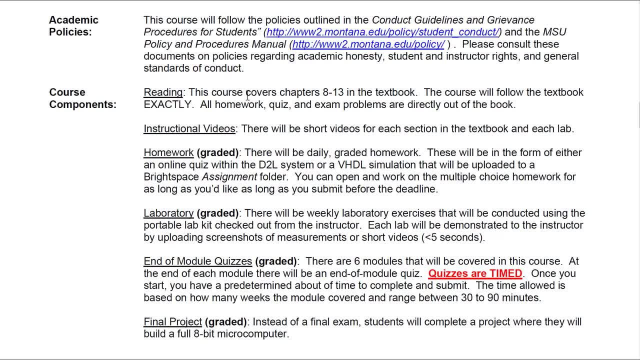 and instructional videos. So this is the way that the information is given to you. Okay, We cover chapters eight through 13 in the textbook. We follow the textbook exactly, So you should be able to open the book up to chapter eight and start working through it And. 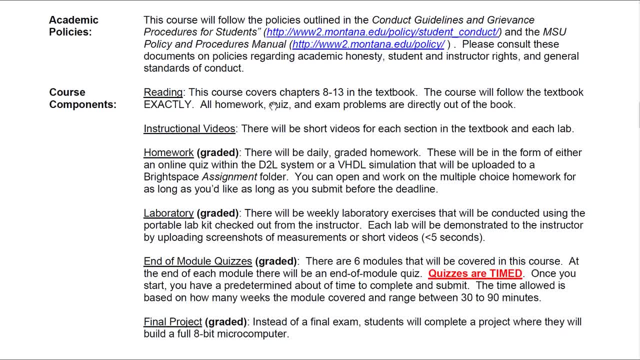 we're going to follow it. We're going to do every section in the book all the way until the end. Every one of the sections in the book has one or more instructional videos. They're all on YouTube so you can. you know they follow exactly. It's just me and both of them. So whatever mode you, 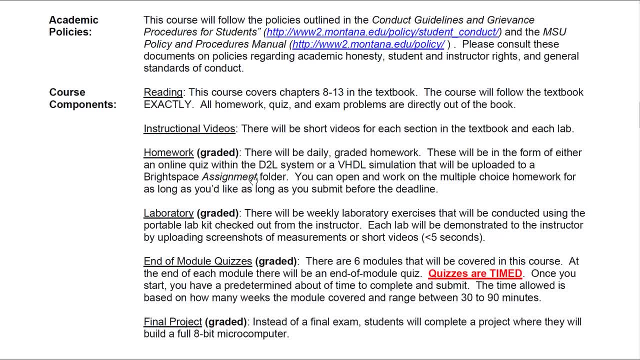 like to use. it's there for you. Then the way that you get practice with the material is through homework. Now homework is graded and there's going to be daily homework assignment And I'll look at every day. You're going to be doing some sort of homework, Okay. Then there's the laboratory. 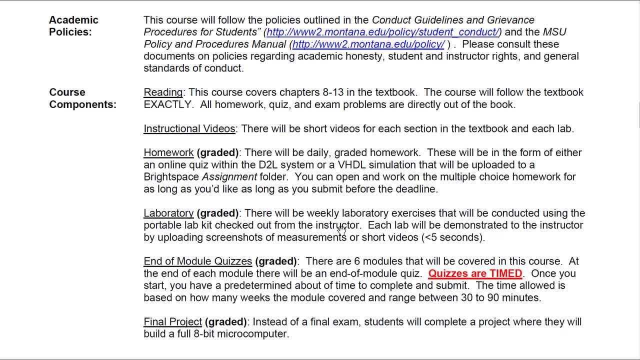 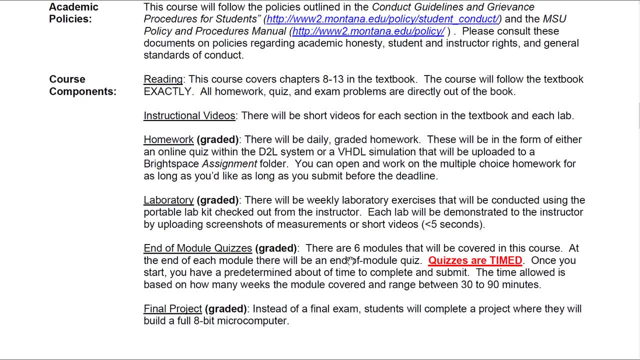 This is also graded almost every day, or every two days. you're going to have a lab and you're going to demo this using, you know, short videos that you upload. Then, of course, you've got the end of module quizzes. Now, the end of module quizzes, the reason that they're a little bit different from 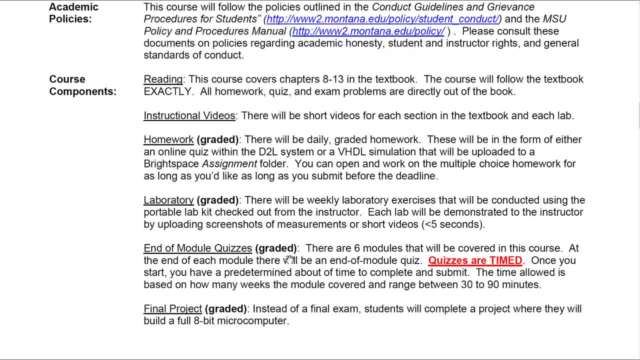 like the homework, even though you might use the same format, their multiple choice format. the quizzes are timed So they're to emulate what it would be like if you sat down in a live class and read it out, a piece of paper, and said go. So you got to have the information in your head. 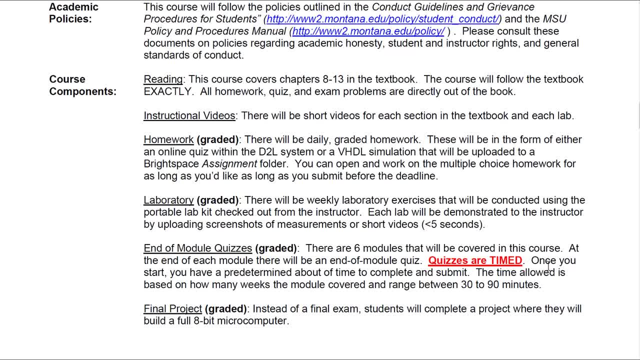 There's not going to be enough time for you to actually scroll through the book and find the answer. You need to study and prepare for these, So they're going to be anywhere between 30 minutes to 90 minutes, depending on the module, But once you hit go, the clock starts and then it ends. 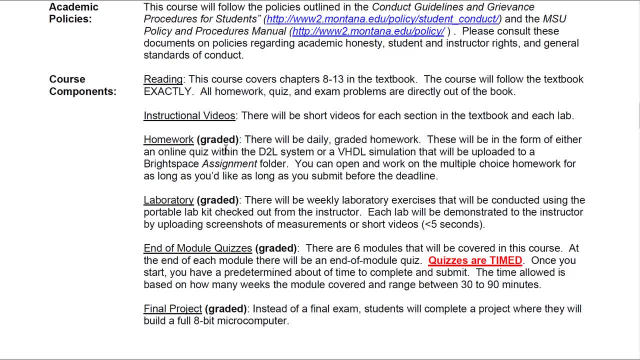 and then you're done. Homework is not like that. If it's a multiple choice homework, you can open it up at the beginning of the class, look at it, You can enter your information, you can save. you can then come back later. 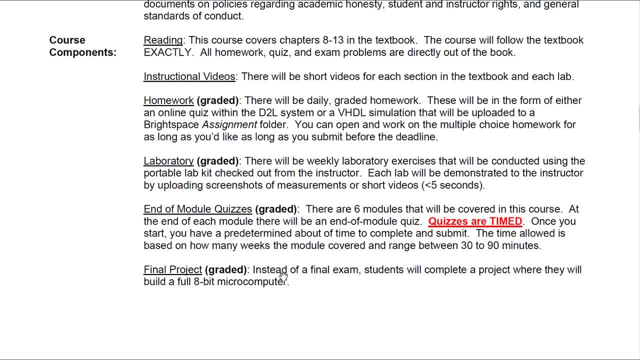 Deadline is the actual deadline for the homework. Okay, And then there's the final project. This is a big one. I'll have- I have a big video of this later in the class that you'll watch- but you're going to just do a whole bunch of really cool stuff to build this full computer. All right, 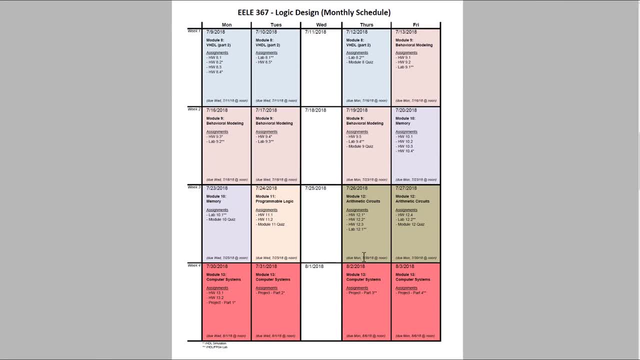 here it is. This is the schedule that you have four weeks. Every day, the class is broken out as if you were meeting Monday, Tuesday, Thursday, Friday. Okay, On every one of these days there's going to be a lot of activity associated with it. 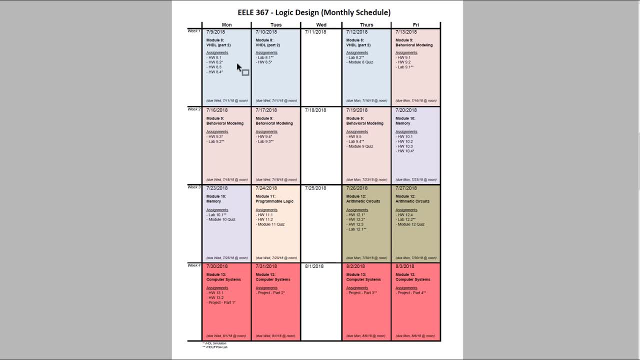 So if you think about a 16 week semester or a 15 week semester, the expectation for a class in terms of workload is a four credit class, or every credit that you take is supposed to be approximately two to three hours of work. So that means you know, for this class let's just use two hours of work. 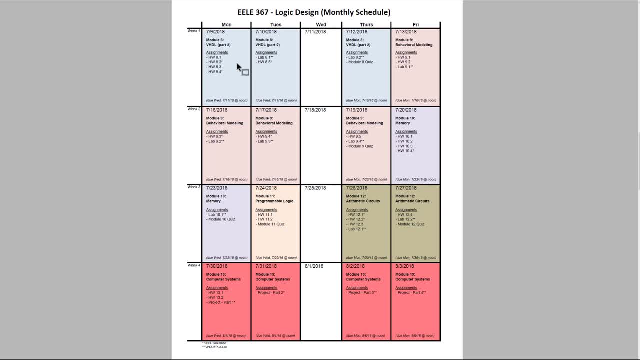 So if you take a one credit class, that's two hours per week that you work on it in a normal semester. So if you took 15 credits, if you think about that, that's somewhere between you know 30 to what. would that be 30 to 45 hours of effort. So, yeah, if you take a 15 credit. 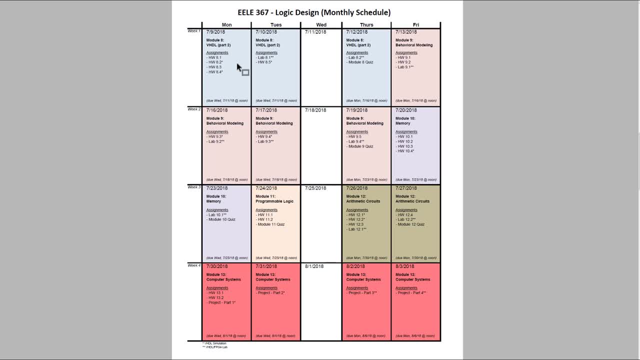 load. you are essentially a full-time employee. It's about comes out to be about 40 hours on average of how much time you're spending. That's right. That's exactly what it is. That's why 15 credits is considered a full-time, a full-time job, Okay. So now let's apply that to this class. 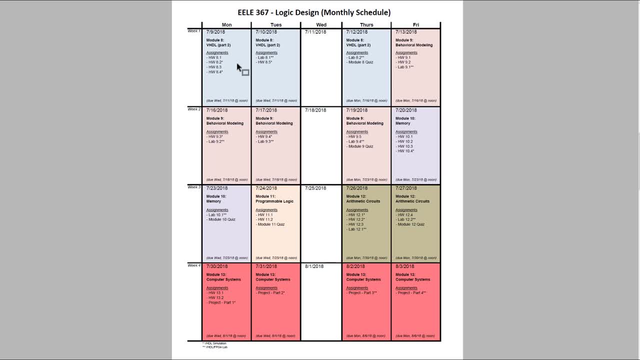 So you have this class right. here is four credits, So you should be spending in a semester, a four-month semester. you're going to be spending four times two to three, So that's between eight and 12.. So let's just say 10 hours a week. So now you're spending 10 hours a week. 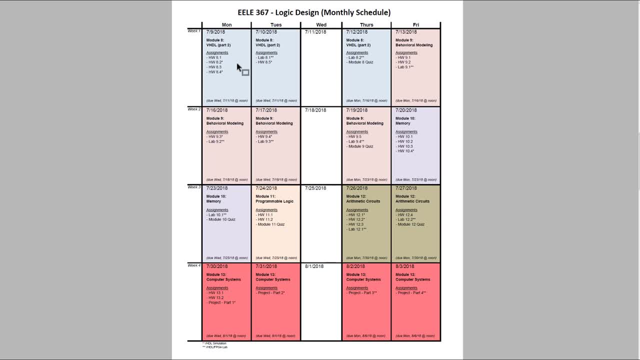 during a four-month semester. Now you're going to compress that into four weeks, Okay, So you're basically going to do four times the amount of work. So the numbers come out to be that you're going to be spending about 40 hours a week on this class. So you should be prepared for that. 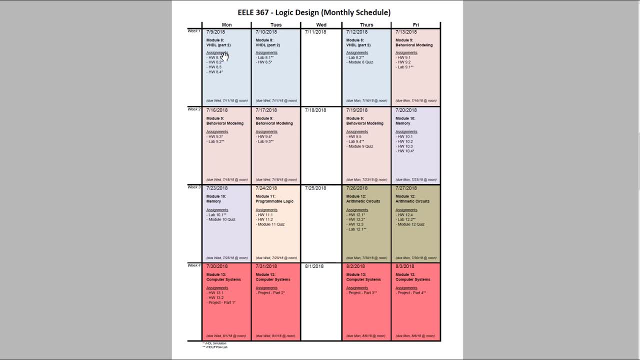 It's a full-time class, So when you think about four days a week, every one of these days is going to be eight to 10 hours of effort, So be prepared, This is a full-time job. What I do is: every day I show. 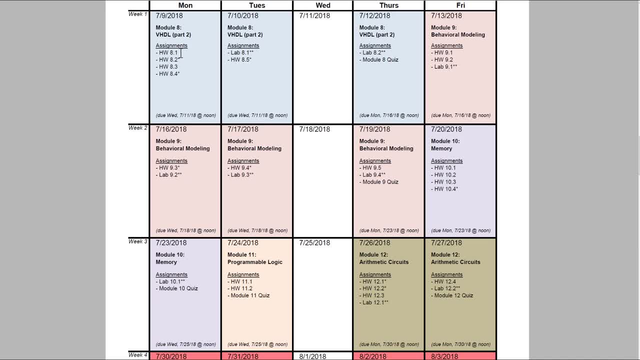 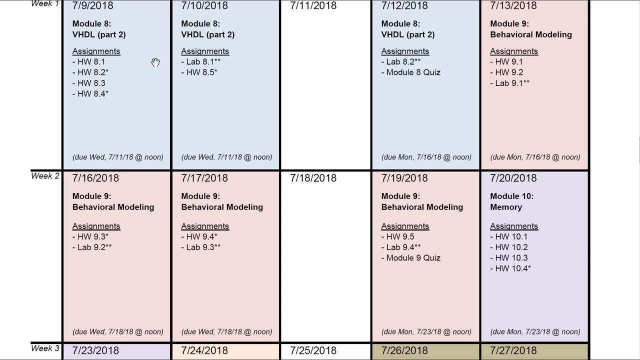 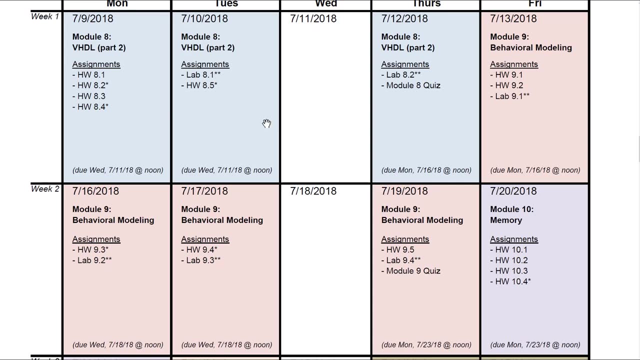 you exactly what the deliverable is. So when I say homework 8.1, that means you have gone in and done the exercises, You've read section 8.1, you've watched the videos for 8.1, and then you've done the homework, et cetera. Okay, So now here is the deadline. So what I 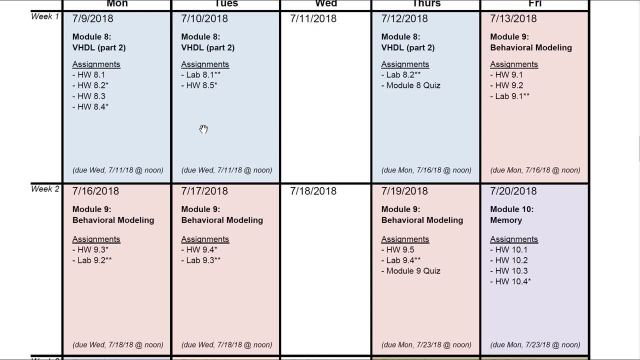 decided to do to give you flexibility, since this is an online class, is the deadlines are. there's two per week, So you're going to have a deadline on every Wednesday at noon which covers the deliverables that were covered on Monday and Tuesday. You don't want to fall behind You're. 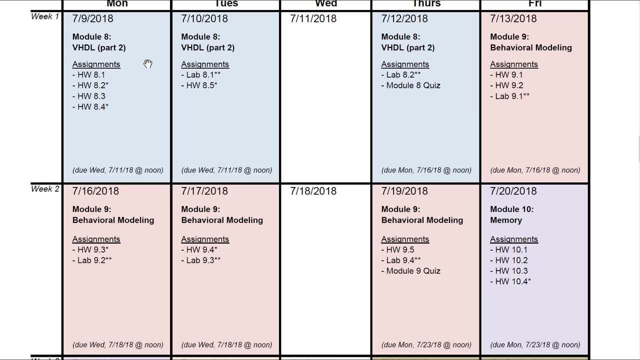 not going to be able to get up Wednesday morning and crank out all the information or all the activities for the Monday and Tuesday assignments, But I do want to give you some flexibility. So if you do get stuck Monday on something, you have time Tuesday morning to get help If you get stuck. 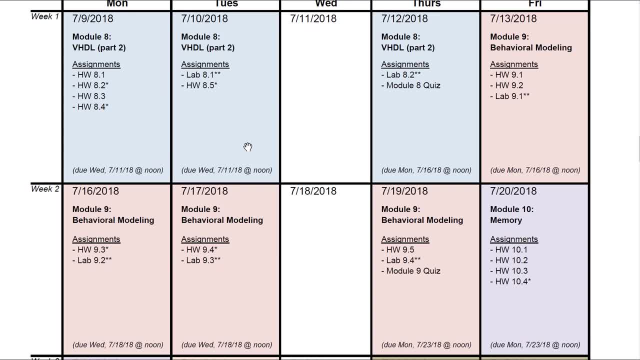 on something on Tuesday. you have Wednesday morning to get help And it just it'll. it gives you a little bit more flexibility, since this is an online class, But Wednesday at noon is the first deliverable of the week. Then you have your Thursday and Friday activities and these ones. 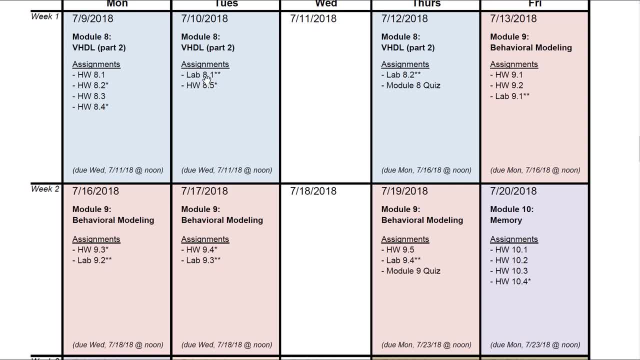 are going to be due the following Monday at noon. Okay, So if you look at these down here, I tell you when things are due. So Monday, everything's due. you know, July 11th at noon. All your Tuesday activities are due July 11th at noon. Wednesday: If you look at your Thursday and Friday, they're 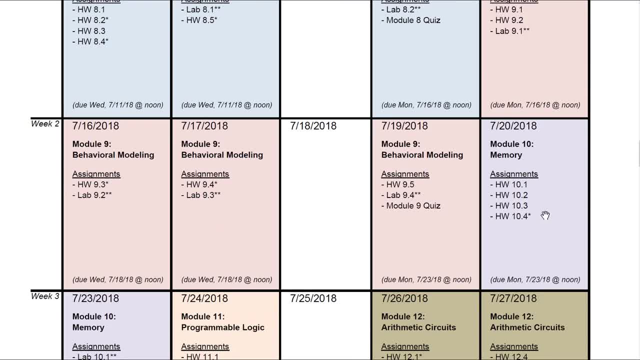 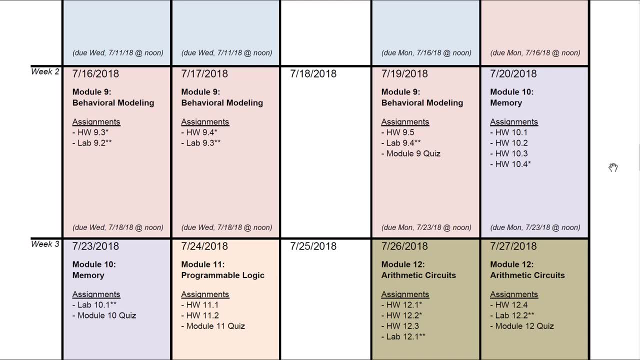 due the following Monday at noon. Following Monday at noon, you go to the next week. exactly the same thing. Your Monday Tuesday activities are due Wednesday at noon. Your Thursday Friday activities are due the following Monday at noon. And you just go and you go, and you go and you get to the end the last week of the 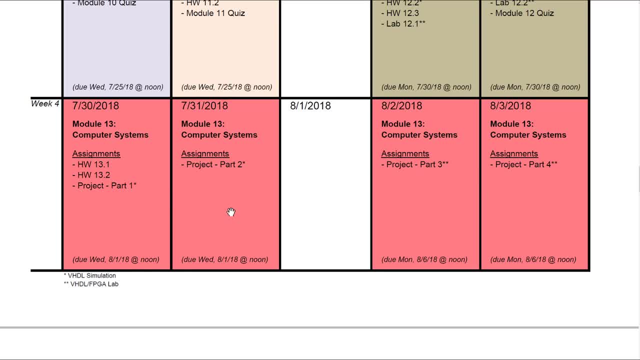 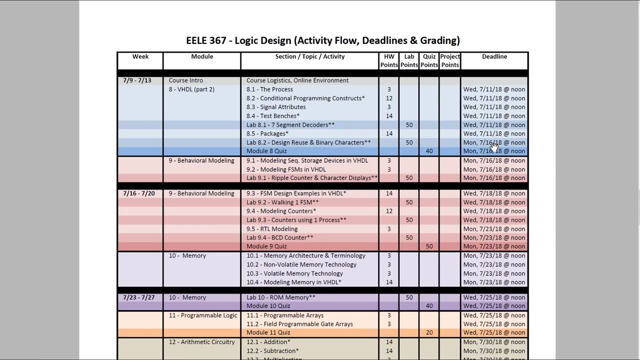 class the full week on building this computer system. Okay, So it's very important to keep track of these deadlines and do not fall behind because it's just there's too much work to get caught up. This is: this is a different view of all the assignments. It shows it to you in like a. 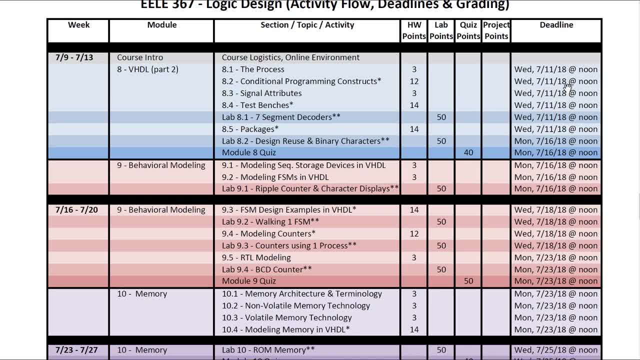 table form. It shows it to you in like a table form. It shows it to you in like a table form, But it shows you the amount of points associated with it, And I did duplicate the deadlines here so you can see what's going on. But here's the four weeks of the class And you'll notice that 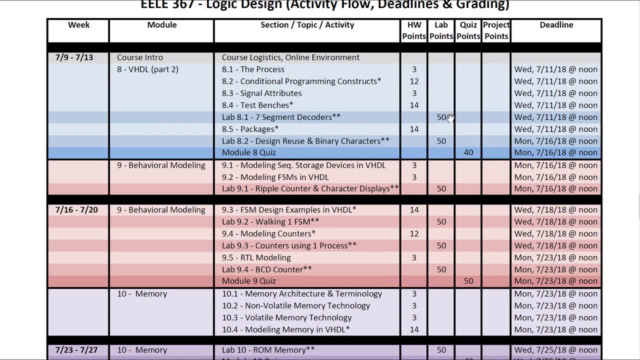 when you come over here. homework assignments are worth certain points, Labs are worth certain points, Quizzes are worth certain points, And you'll notice that the labs have a lot more weight to them. Okay, So these are 50 points for a lab on 8.1, versus a homework which is due or which is. 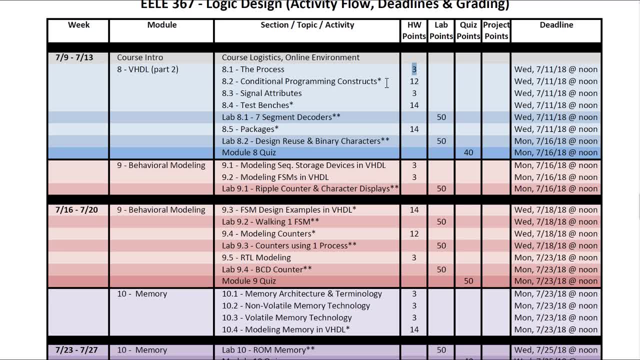 only worth three. I also made a note on here which homework assignments are going to be VHDL assignments, And you'll notice that those are worth more points than the multiple choice quiz format homework. Okay, So you can actually walk through here and you can, just as you, knock these. 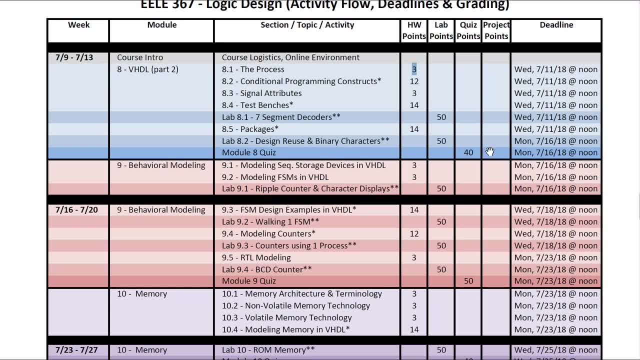 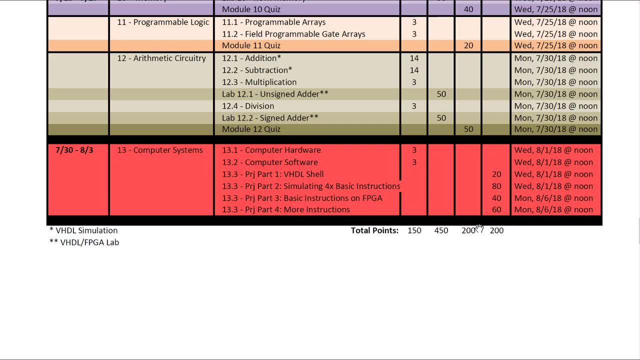 off in Brightspace and you get graded, you'll be able to see your points just accumulate. Okay, And so you go all the way down here. Like I said, here's the totals for each of the categories. These add up to be a thousand points. Okay, Then, if you're curious about why we're doing this, 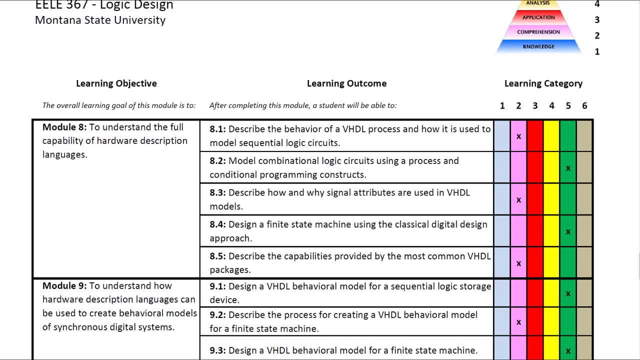 you know, everything we do in our college classes is for something specific. We're trying to learn something specific. So I actually put down here, I'm going to put down here, I'm going to put down the specific learning outcome for every section that we're going to cover. And I give you a little. 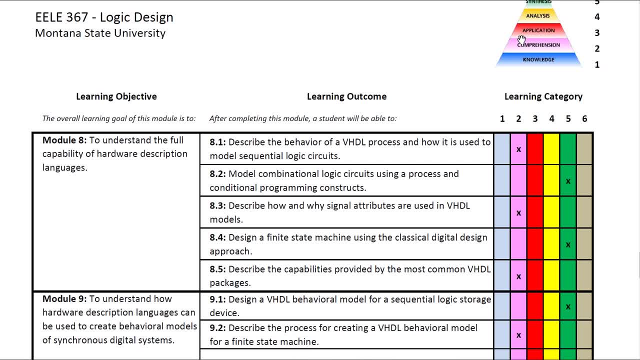 bit of you know Bloom kind of Maslow's hierarchy here or Bloom's taxonomy, in terms of what level of learning you're doing. So there's low level learning, like knowledge and comprehension, where you're just like learning something, just getting facts and figures together. Then there's 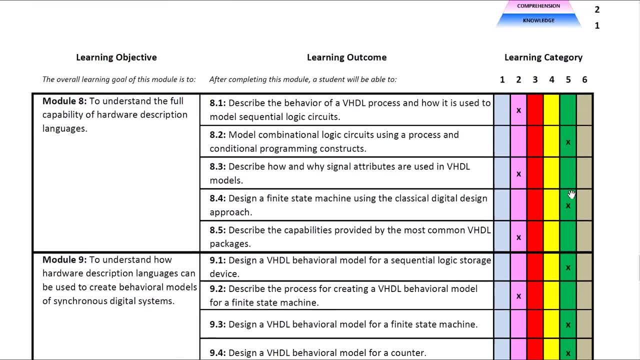 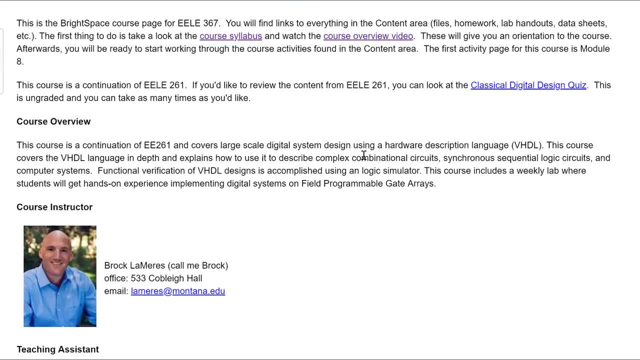 also pretty high level modes of learning where you're actually designing something. Okay, So I just call those out if you're curious why we're doing this. Okay, So that's the syllabus. Now let's look at what this course is going to look like when we get into the content. So if I click 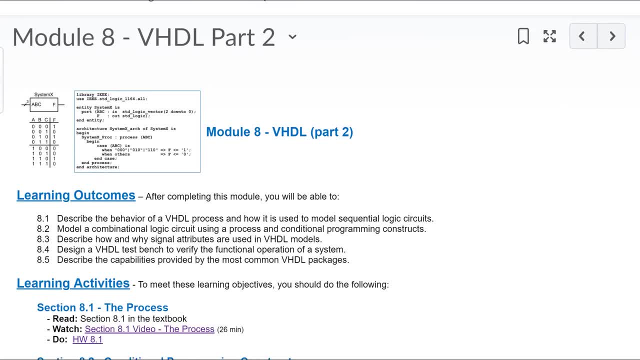 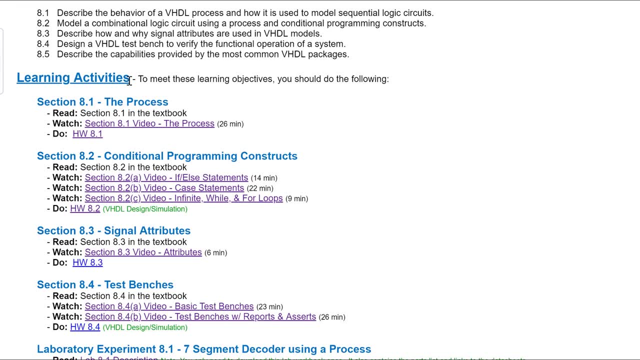 this arrow, I go over to module eight. Every module has this same format. You're going to have the learning outcomes. That's why what we're going to learn when we do these activities, And you're going to have activities broken out by the section. So in section 8.1, you're going to read the 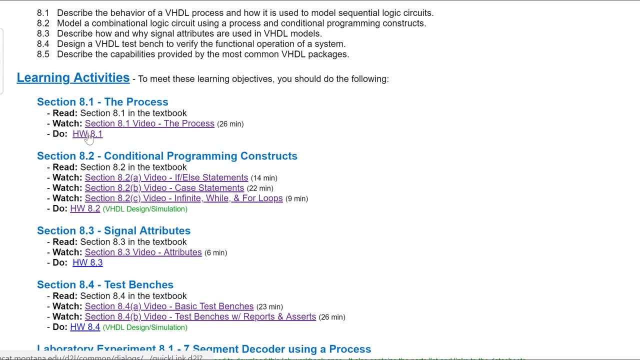 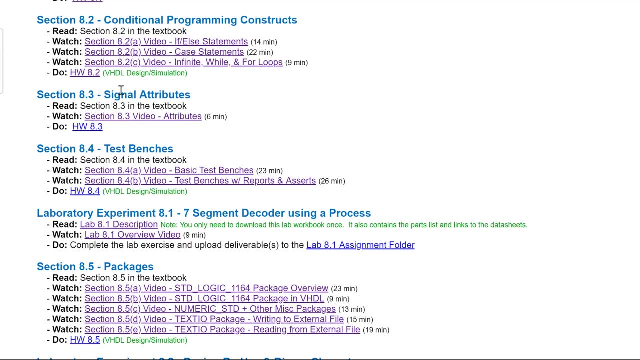 textbook. You're going to watch a video and then you're going to do the homework. 8.2, same thing read in the textbook: watch multiple videos this time and then do the homework 8.3,. guess what. 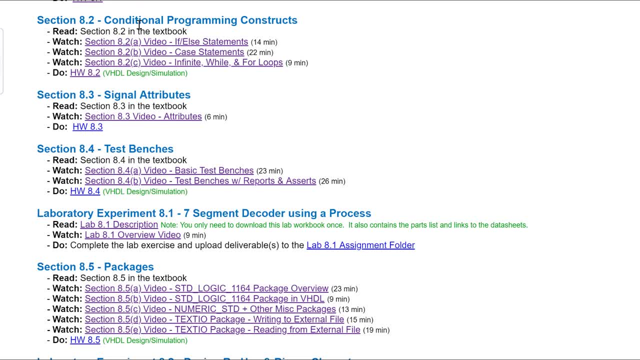 Watch the videos, do the homework, Repeat Okay. But then, as they go along, after you get through certain sections, you'll end up having a lab video or a lab assignment, where then you'll actually say, okay, I've learned all this content, I've done the homework. Now I'm ready to build some. 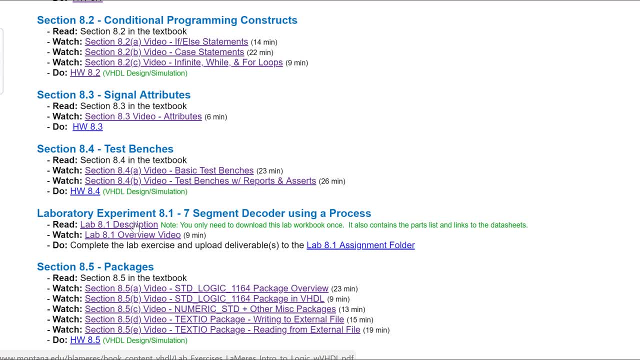 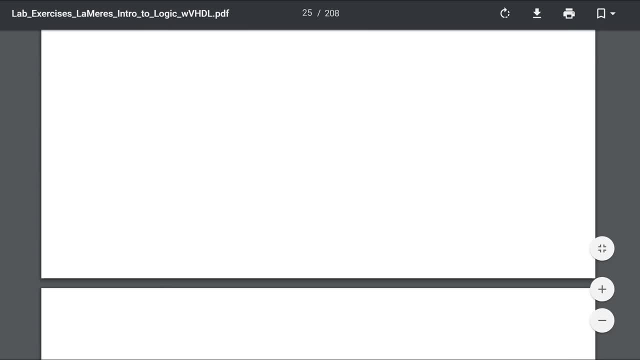 circuits. So what you're going to do is you're going to click on this lab description and it's going to download this big lab manual. You only need to do this once. It's a big PDF, but you'll go through and you'll read the lab assignments in here and you'll see what you're actually. 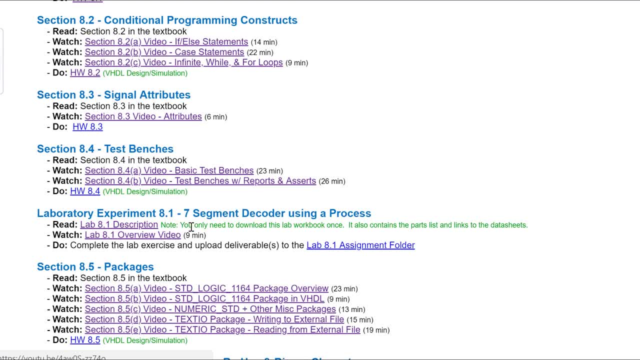 doing, And then I do give you a video on all of them, And then, when you do the lab, you're going to have these deliverables. So the videos and the screenshots, you need a place to put them, So you're going to upload them to the assignment folder. Okay, So that's how this goes. And then 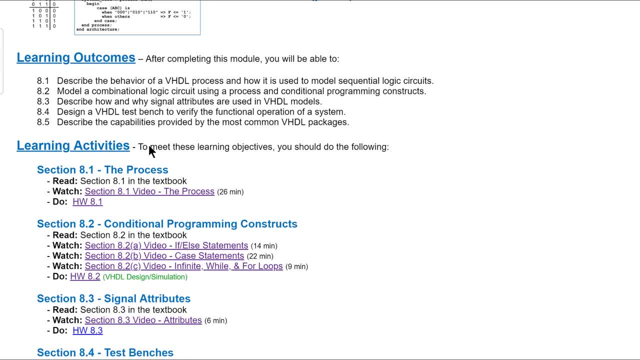 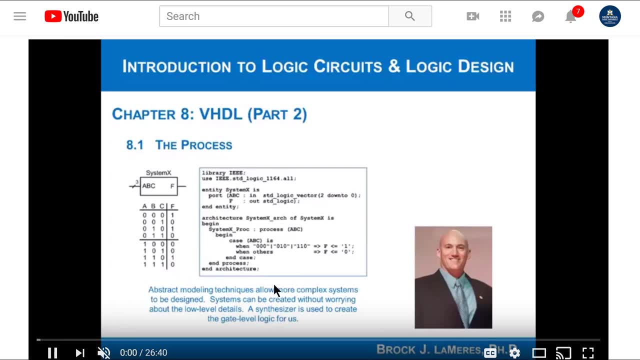 each module has an end to module quiz. Okay, So when you click on these things, if you look at it like when you click on one of these videos, it's going to take you out to YouTube. Now watch the sound here for a second. It's going to blast. Okay, I got the sound muted, So it's going. 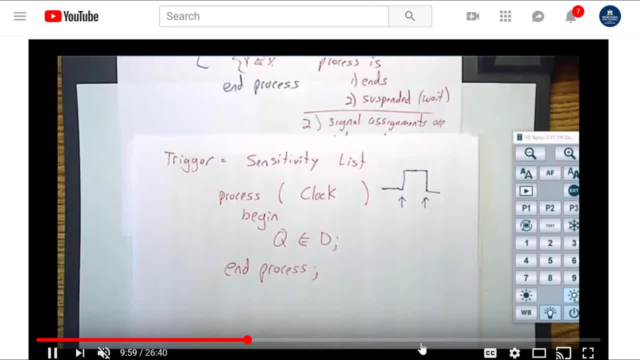 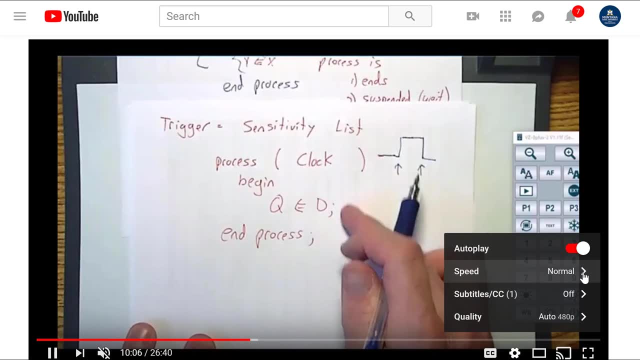 me doing stuff like writing on paper or you know writing code or whatever, And so you just watch these videos on YouTube. If they're too slow for you, you can speed them up, You can do the settings to to go a little bit quicker And that's the the videos When you click on like the. 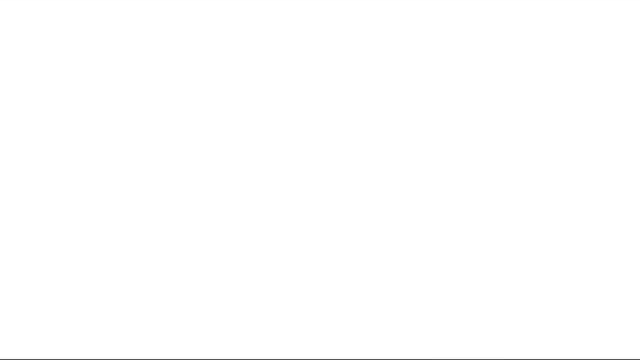 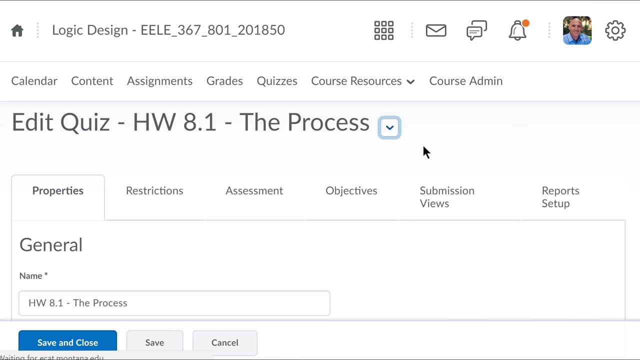 homework. what's going to happen is it's going to open up the quiz tool. Okay, So this first homework is a multiple choice quiz. So you come in here and, like I said, this looks a little bit different, but it'll come open and it's just like a normal bright space. 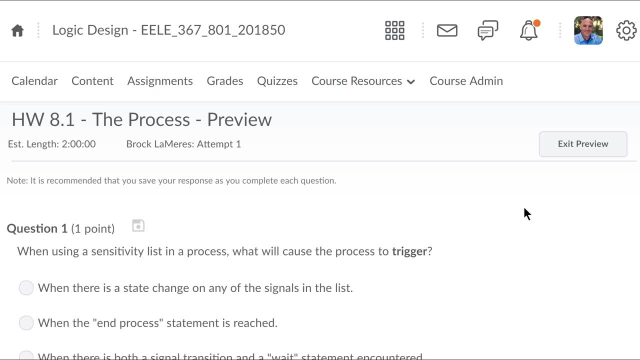 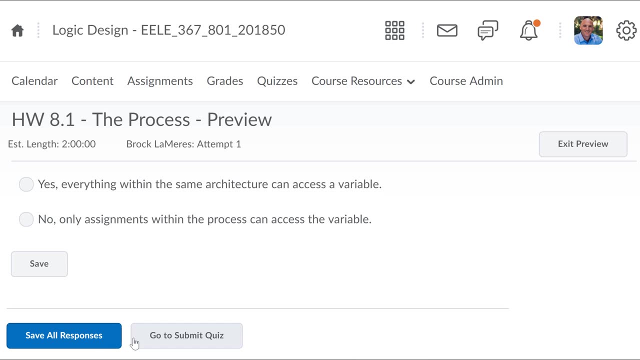 So you come in here and you're like, all right, here we go Quizzes. All right. When using a sensitivity list, what will cause the process to trigger? You enter your answer, you go down, you got to make sure that you make sure you can save and then wait until the deadline before you. 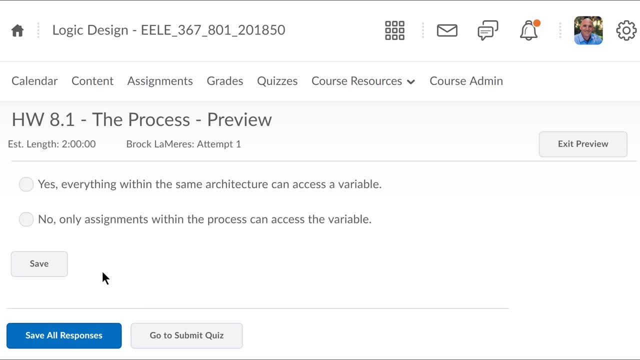 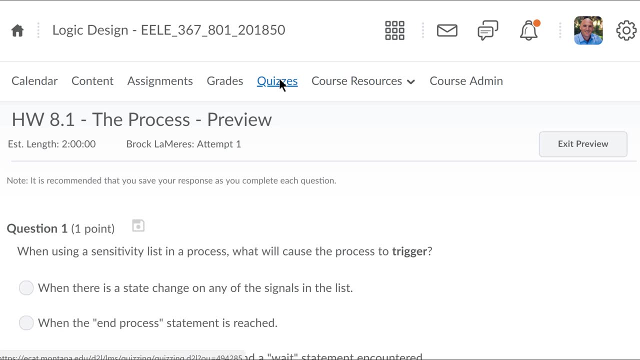 submit, or you can go ahead and submit it. It'll give you your grade immediately And then it'll enter into the grade book immediately. But the cool thing about it is that you could go to the quiz tool and actually look at these quizzes and you can see all of them at once of where you are. 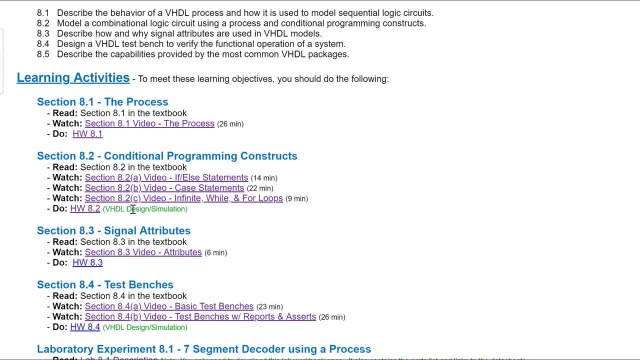 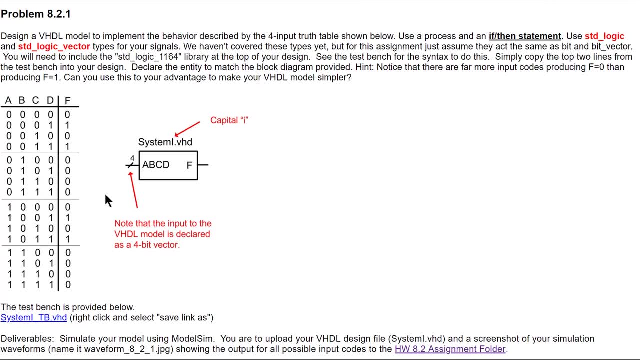 is linked in the content. Same thing when you have a VHDL design simulation. when you go to do the homework, it takes you to a webpage and it's going to define the problem for you And it's going to give you anything you might need, like the functionality or the test bench. Then it has a 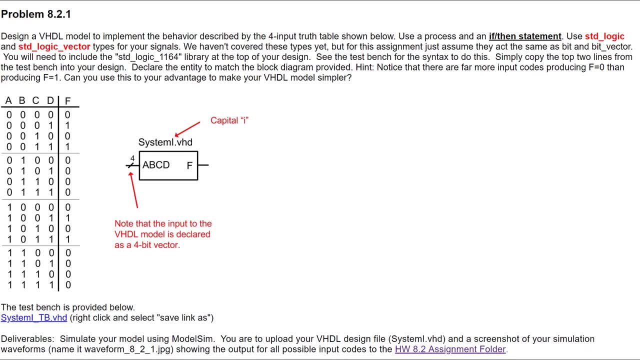 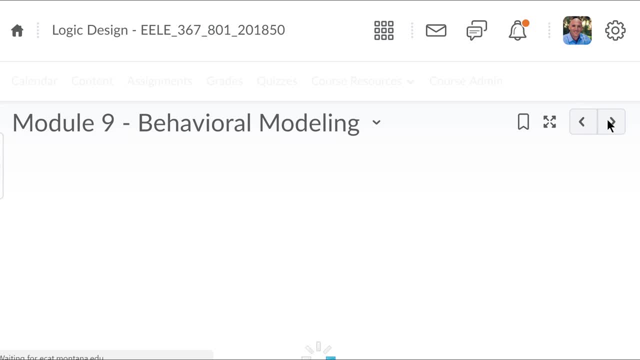 link to the assignment folder. So you click on the assignment folder. it'll take you to a place where you can upload your files. Okay, So that's a module. The good thing about it is that it's all designed where it's all the same look and feel. So you go to the next module. guess what? Learning. 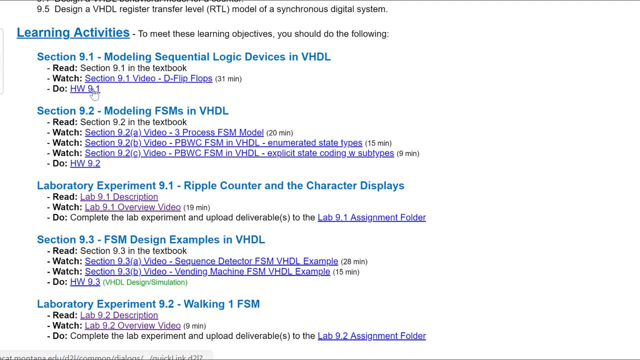 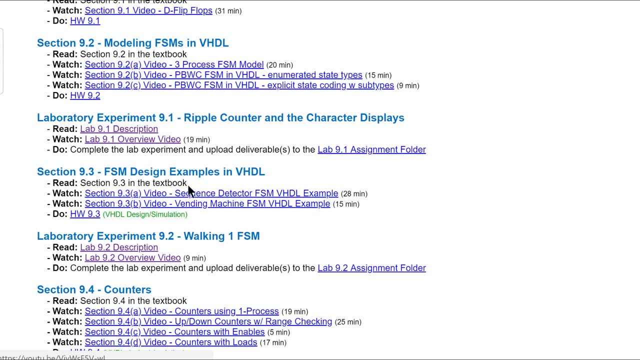 modules are just the same thing: Read, watch a video, do the homework. read, watch some videos, do the homework. Oh, and that's time for a lab. Read the lab description, do the video or do the assignment. And you just repeat, and repeat, and repeat, And you go through all these things and 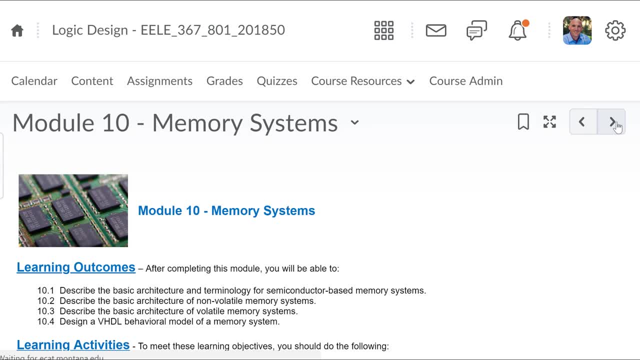 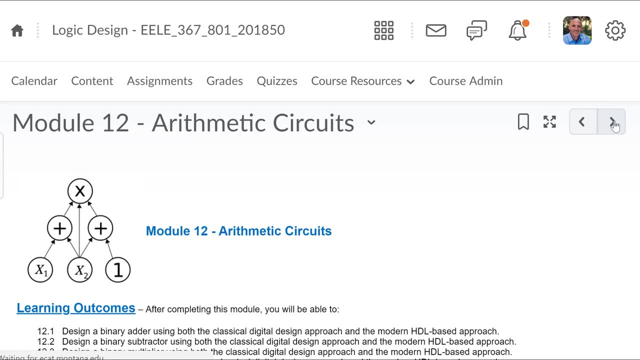 then the course will be over. Now you get to the last component of this course is this computer project. The computer project is the grand finale, right? So it's this huge amount of effort It's going to bring everything together. So I have a pretty large, not necessarily too large. 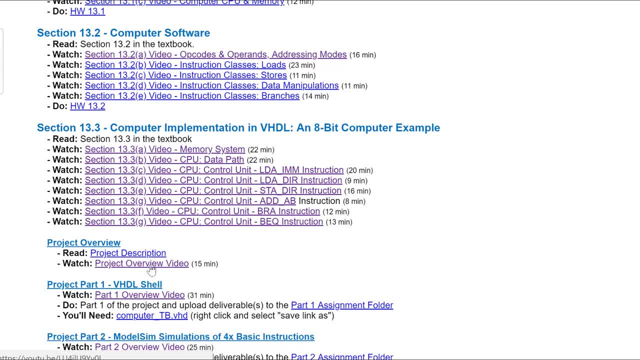 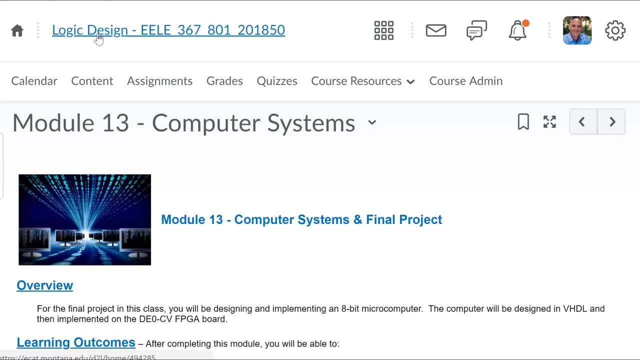 but I have a lot of videos to watch here and I give you a project description of this and this will be kind of the great moment of the class. Okay, That is it. So at this moment in time, you are prepared to start doing this course. So the first thing you're going to want to do,